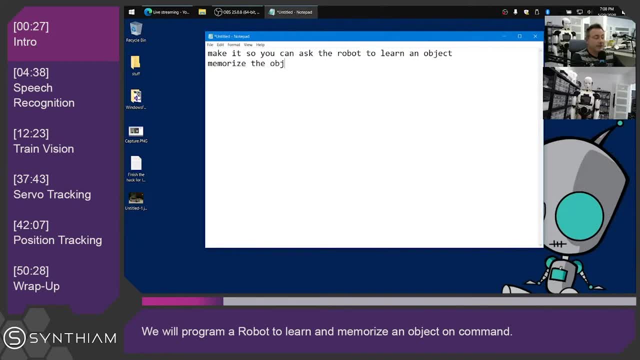 And then it'll memorize the object And then, when it sees the object, it'll say what it is Okay, And you can do this. So we'll essentially loop this, So we can do this a bunch of times, All right. 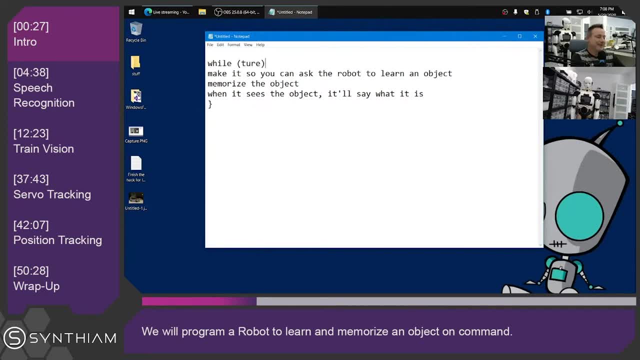 So there, Oops, Okay, And that's essentially what we're going to do, So we can make a quick project. We'll do it on my computer, first on my laptop, so you can see everything I'm doing, And then, once we get it all set up, we can save the project. 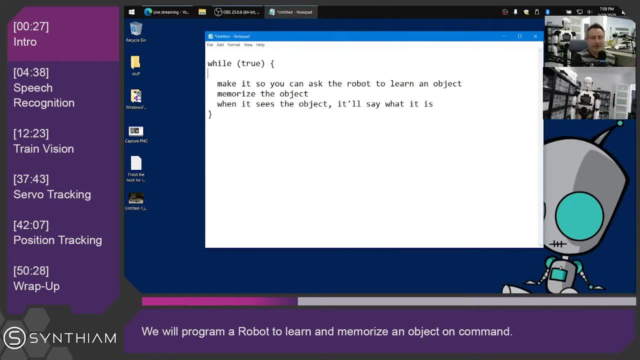 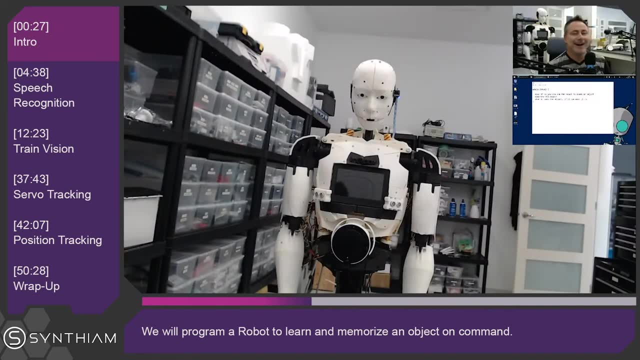 and import it into the InMove which is behind me And we'll use the InMove which is actually on. He's just not doing anything right now. We'll use him to learn the objects and then, like, maybe point at them or something like that. 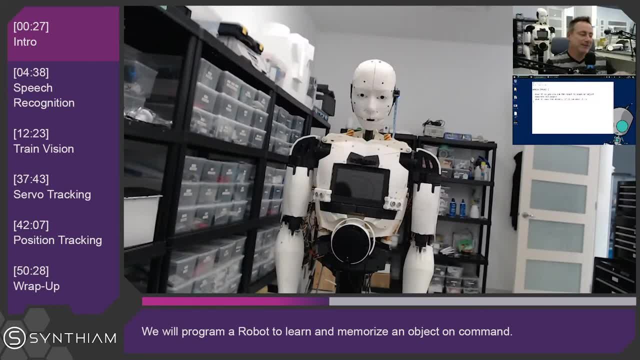 It'll be fun. I don't really use the InMove very often, but we started to use them just recently And I'm a fan. I really do like the InMove. It's pretty cool. So how are we going to do it? 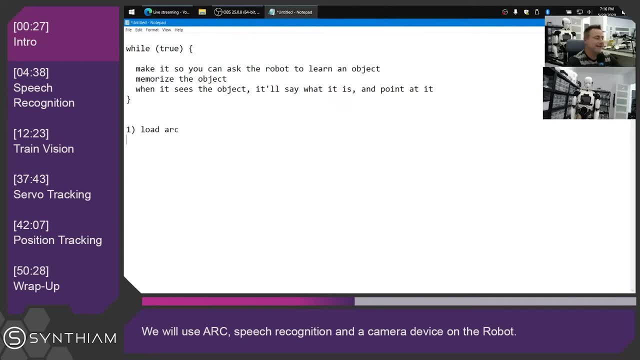 What we're going to do is we're going to obviously boat arc And we're going to use speech recognition And we'll add a phrase, And the phrase that it's going to detect is going to be something like learn a new object. 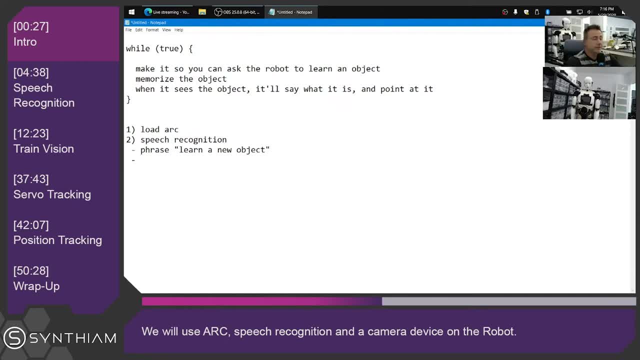 Okay, And then what that's going to do is it's going to ask what the object name is, And then we're going to use Bing speech recognition, And this is from Microsoft. This is using the Azure, Microsoft Azure Bing speech recognition. 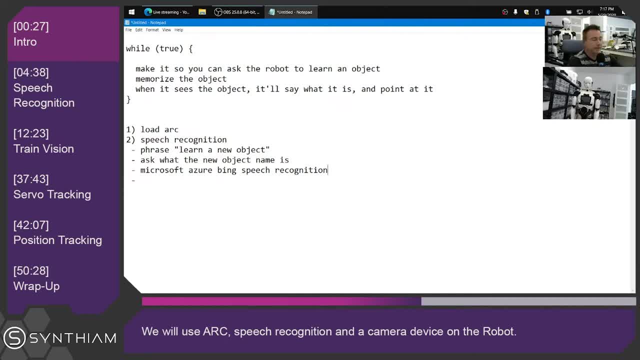 And then it's going to ask it's going to use that and it's going to say it's going to grab the variable essentially Okay. So we'll just say like object name, And then that object name is going to. 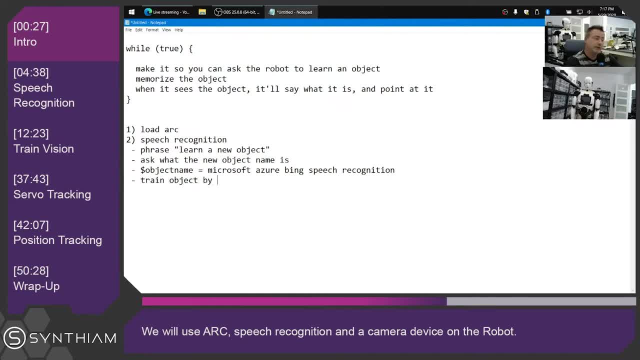 we're going to use a plug-in called train object by script, I think it's called This is a robot skill And it's going to take the object name And then we're going to you know. before that, I think. 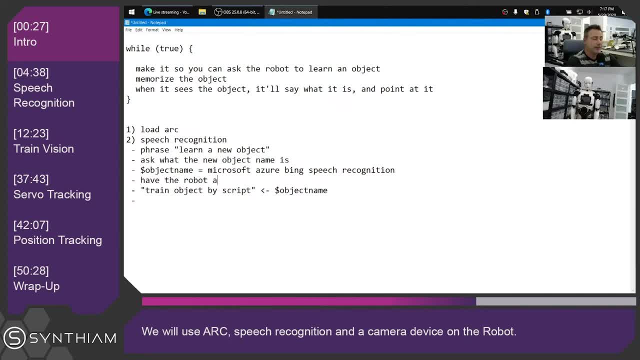 what we'll do is: we're going to have the robot ask: let me know when you're ready. So the robot. we want the robot to give us some time so that we can get the object in front of it and be all prepared, right? 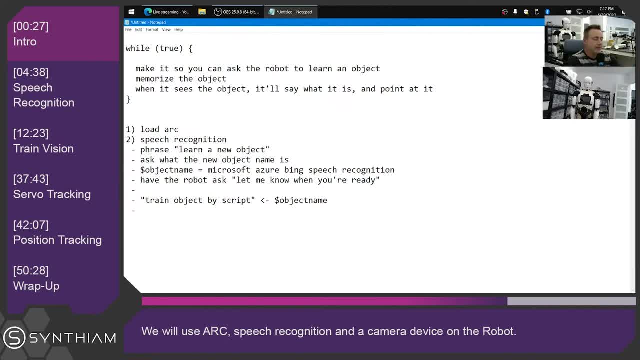 So let the object know when we're ready And then it'll wait for speech, So something like us to say okay or cancel Okay, And then it'll run the train by script. Essentially, what we'll do is we'll hold the object up. 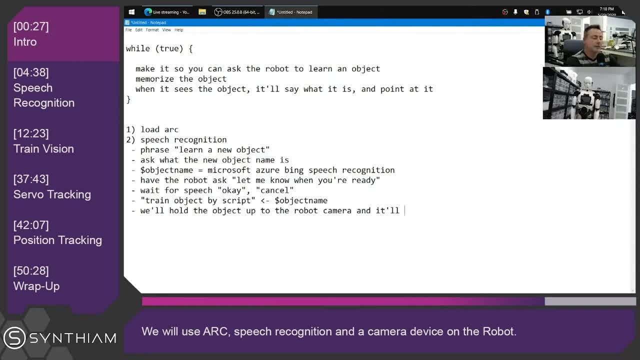 to the robot camera And it'll learn the object. And then what we'll do, that's all going to be started from the speech recognition And then what we'll do is we're going to, I guess, in the camera device we're going to make it so that when tracking, 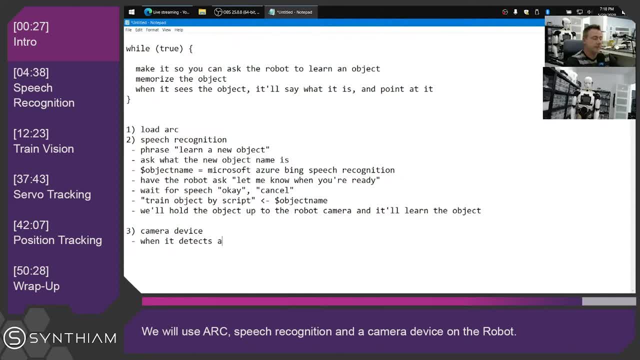 when it detects an object and tracking starts. we're going to have it speak And say I see an object And we'll put like whatever that object name is right. We'll say I see blah, blah, blah And then that's it right. 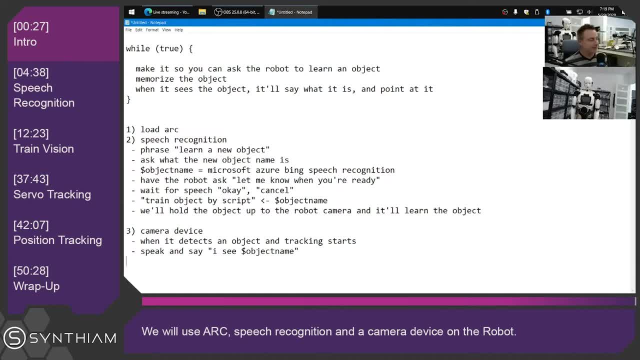 It doesn't sound like a lot, but I mean, when you think about it like in the grand scheme of, like what robots can do, it's pretty cool. So let us begin. I'm going to load Arc And I'm going to set this up on my laptop. 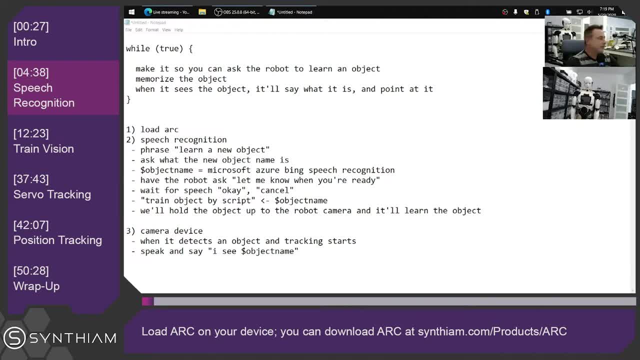 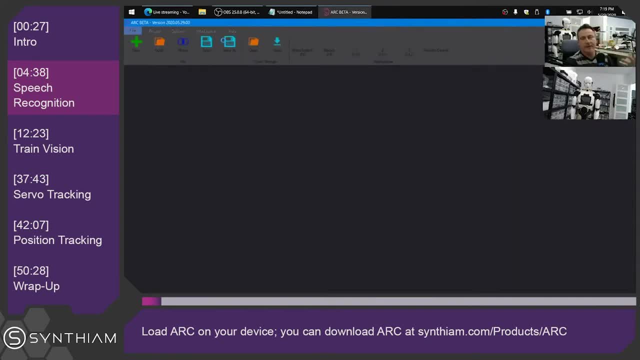 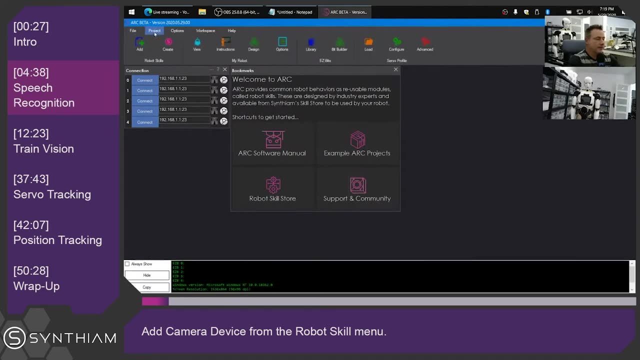 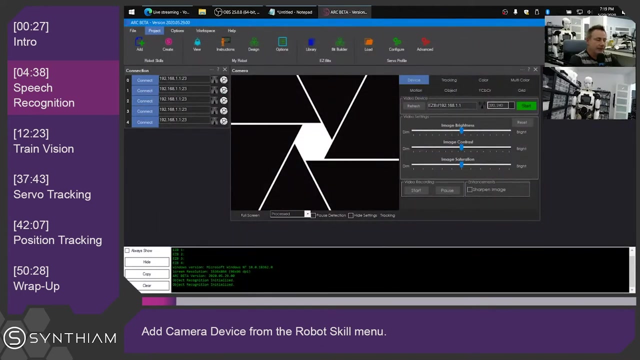 And what we'll do is we'll use the camera that's on the on the InMove And then we'll merge this project from my laptop to the InMove when it's ready. So we'll start by adding a camera And the InMove has a camera. 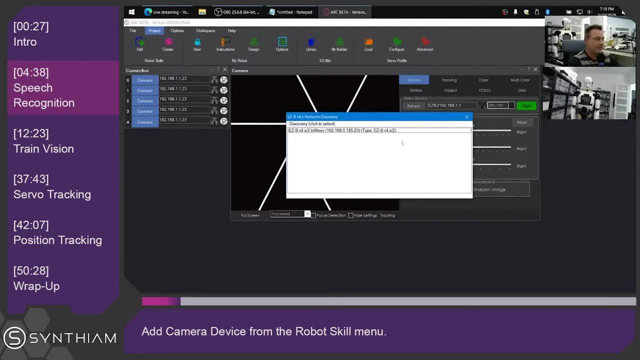 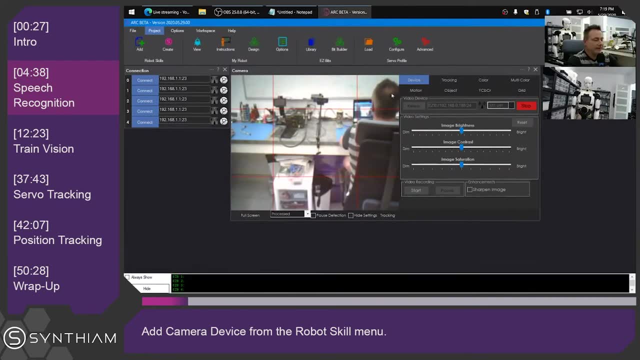 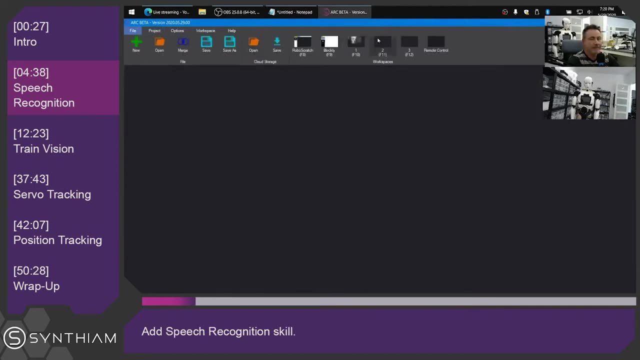 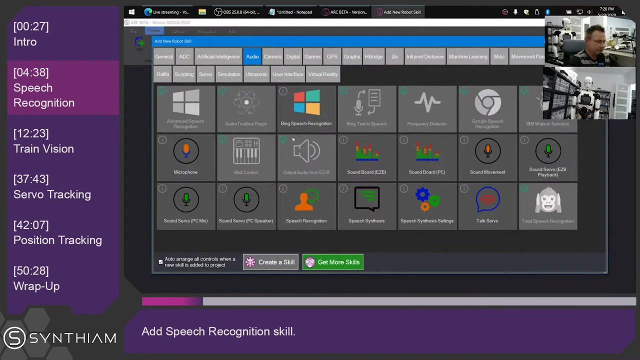 So let's scan the network and find that camera There. it is Awesome, I can see. Now let's move the. we'll just move to the second desktop here And we're going to add some speech recognition on the second desktop. 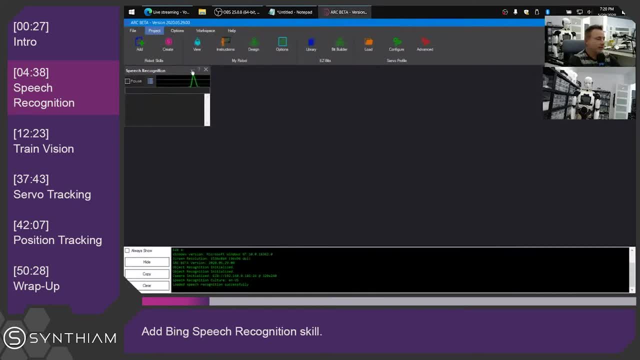 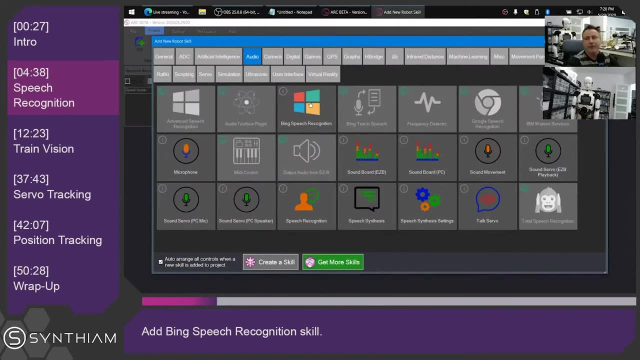 Speech recognition. where are you? There, we are. And then what we need is the Bing speech recognition, This one, So we can use Bing That allows us to use- like I forget what it is like a thousand commands a month, or something. 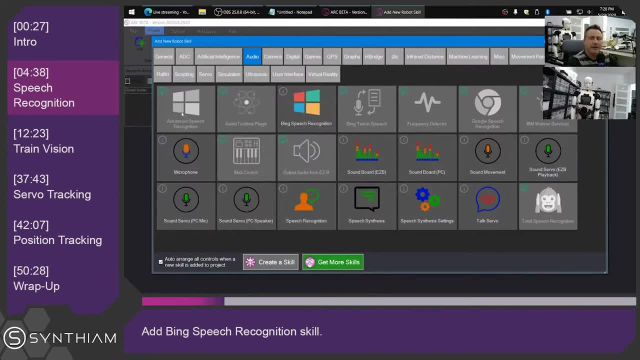 whatever it is, or X number of commands per day. And then there's advanced, which means, if advanced is, you want to set up your own account with Azure and pay it for yourself, you can do like unlimited. well, unlimited as much as your credit card allows. 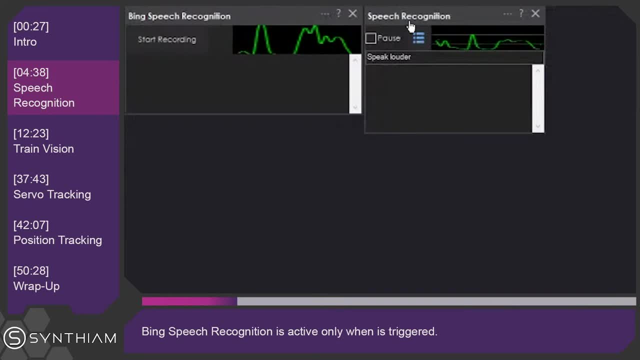 So we'll use Bing speech recognition. So the reason why we're using either of these is because the Bing speech recognition, if it were to listen all the time, it would get really expensive. So we can trigger Bing speech recognition by pushing this button. 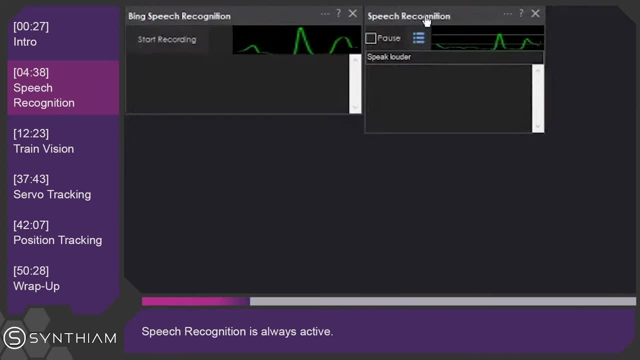 or we can use a control command. So speech recognition- this one is always active. This is using the windows internal speech recognition system, which means that it'll always be listening to whatever I'm saying, And that will be very good for us. 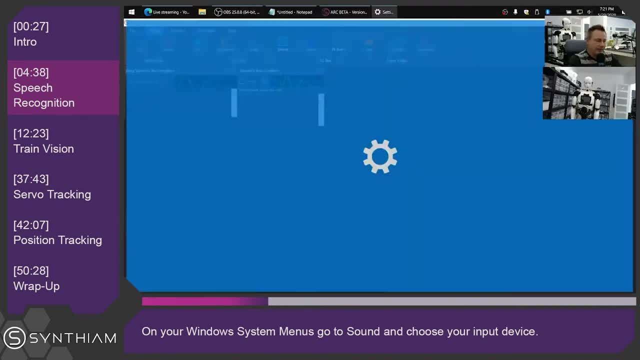 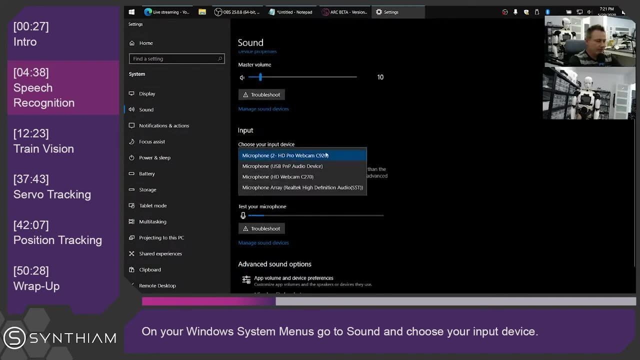 Now let's just make sure that my the, the system that we're using for recording. choose my microphone. It says it's using HD pro webcam. That's probably not what we want. I think we want to use this microphone, Is that not it? 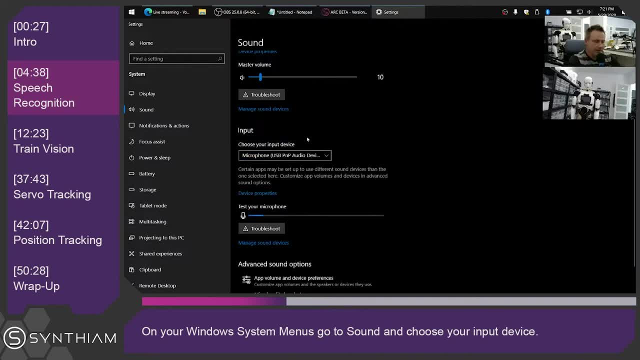 No, maybe this one. There we go, Yep, That's the one USB audio device. Hello, Hello, Yep. So that way it's using the microphone I'm talking into, rather than trying to use some random, because there's so many microphones. 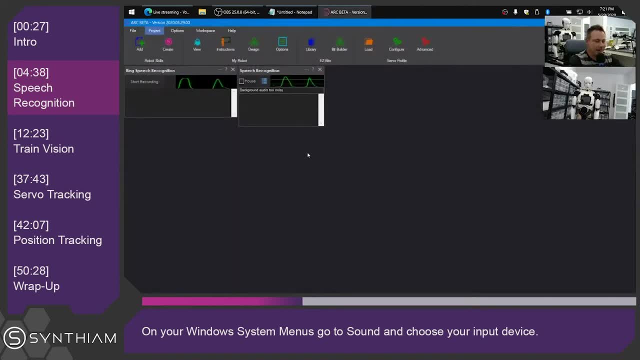 all these cameras have microphones, So I don't think this switches in real time, does it? Hello, Hello, Testing. This is going to be really loud on your ears. It seems like it does. Yeah, Okay, So it seemed like it switched in real time. 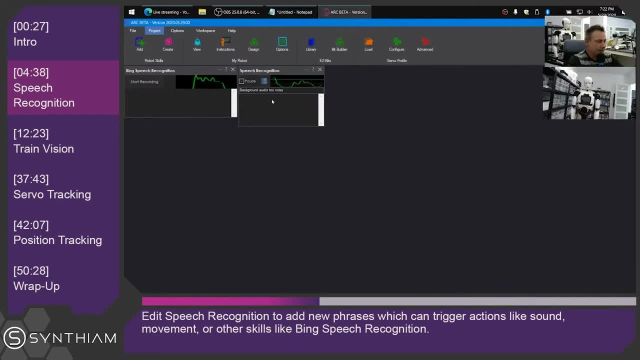 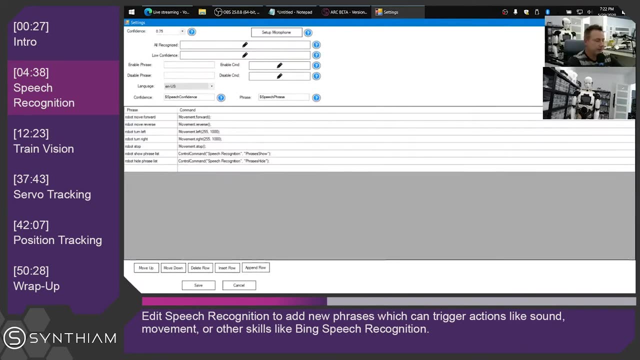 So that's good news. So what we'll do now is we'll edit the speech recognition here and we'll add a new phrase which is going to be learn a new object. So that's the phrase that when the robot hears it, when the robot hears me speak, 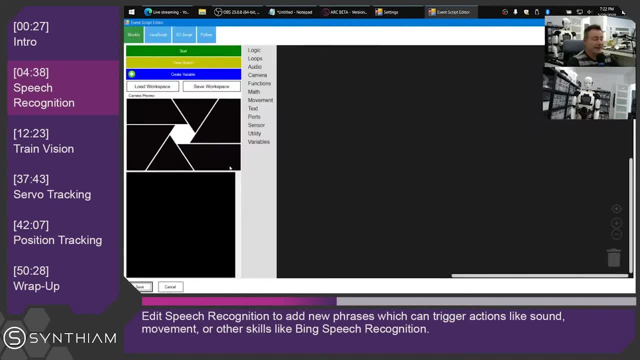 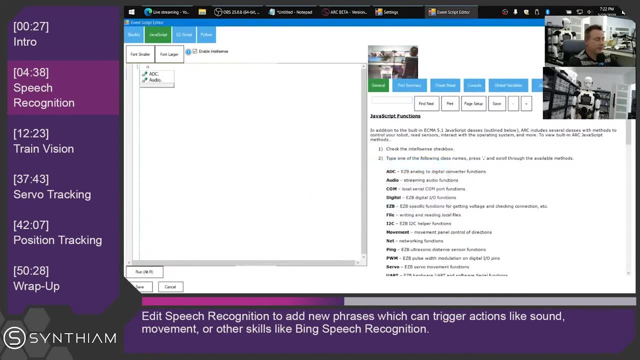 it's going to execute this code that we're going to add. Now we're going to write some JavaScript, because JavaScript is great. The first thing I think we should do is have the robot speak. So we'll go audio dot, say, and do we want it to come out of the easy B? 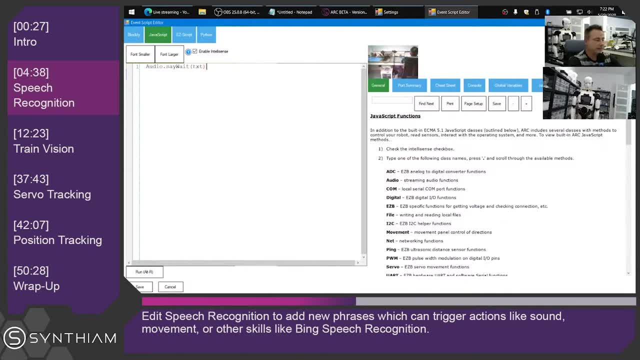 I don't think it's necessary. Let's have it just come out of the out of the PC speaker And I'm going to have the robot speak and say: okay, what is the name of the new object? So it's going to say that to me. 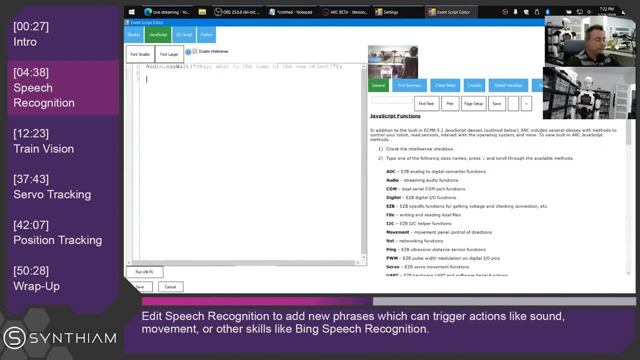 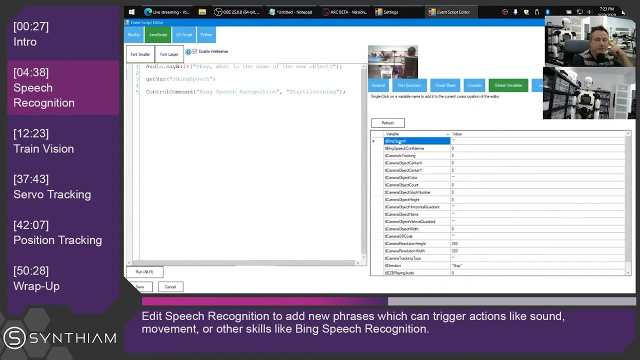 And then what we'll do is we can launch the Bing speech recognition. We'll tell it to start listening And before we start listening, if we look here, the Bing speech recognition will put its response inside of this variable here called Bing speech recognition. 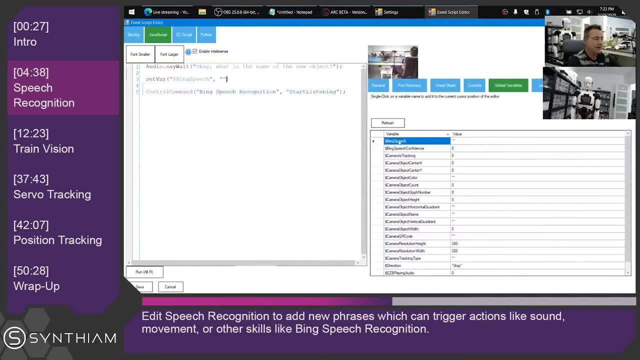 So we can do is we can actually set this variable to empty. So therefore, if anything's ever in there, it'll always be empty, And then we'll do is we'll tell it to start listening And then we'll loop forever while the speech recognition is empty. 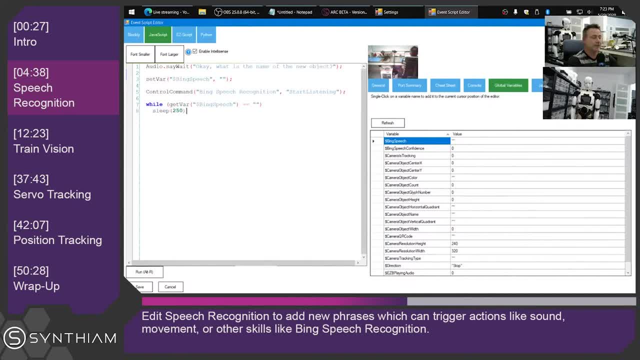 And then we'll just like sleep, for you know 250 milliseconds or something. So essentially, what we're doing is we're just saying: cause that whatever the speech recognition hears like in the in that module here is, it's going to put that phrase inside of this variable. 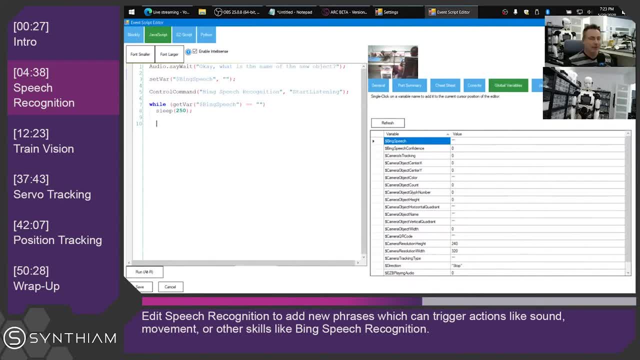 So we're just going to keep looping and not do anything until that variable is populated, Cause once it's populated, then it contains whatever it was that we said, right? So that's one way to wait for the speech recognition to finish, And then what we'll do is now that we have that variable. 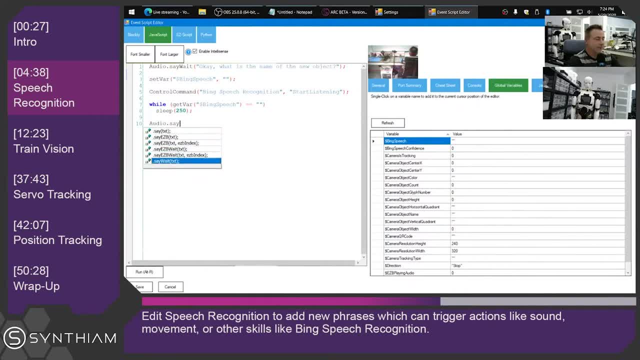 we'll speak again and say: and we'll wait until it's completed and we'll say: you know, excellent, Let me know when you are ready to learn, are ready to teach me? to teach me the- that's the right grammar here. 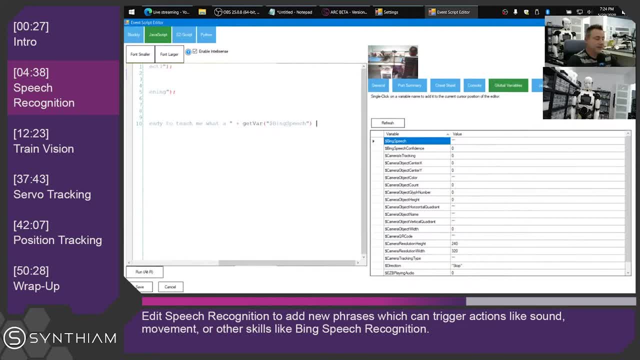 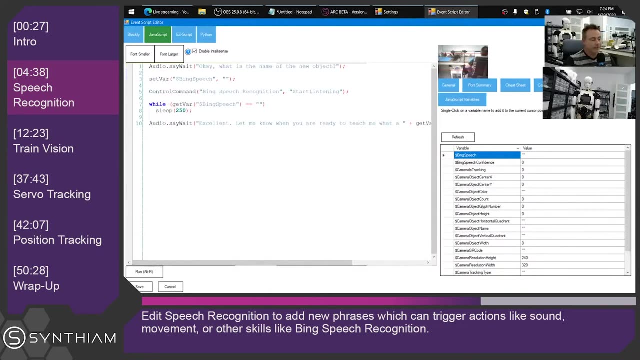 What a, and then we'll put that command, that variable is okay. So here I'll slide this over a little bit for you so you can see whatever. So after, after we get that command or we get the name of the object. 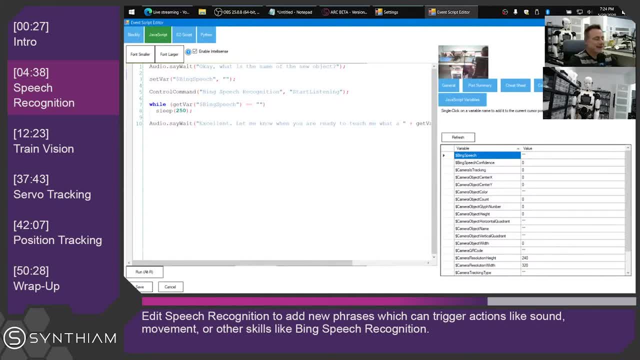 we're just not the robot- interact with us, add some sort of like personality to this whole process And we could, you know, maybe later- I doubt tonight because I don't know if I had the energy, but, you know, another time we can get dive into using one of the aiml or 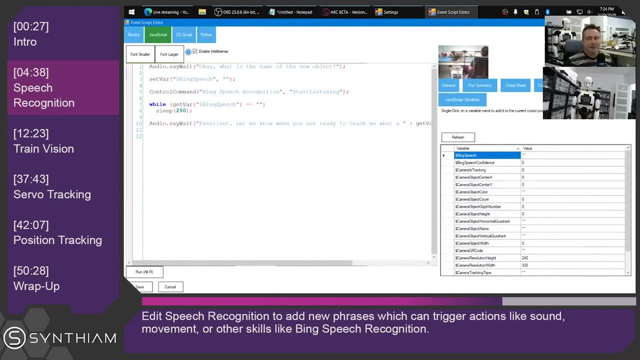 NLP- like the natural language processing, to be able to narrow down exactly and have a conversation, dialogue and get exactly what it is that you're saying. That would be actually a lot of fun. I'm going to make mental note. NLP. 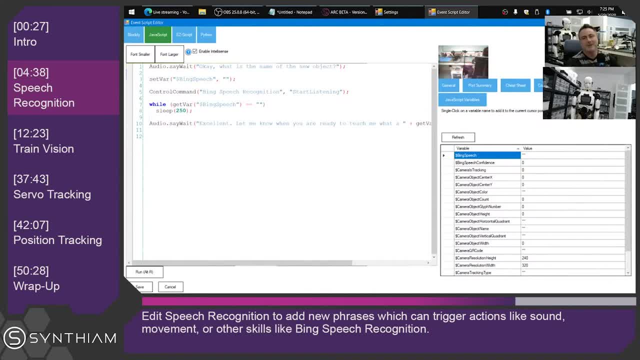 Mix Live hack or one of the future ones. you guys let me know, Um, Um, okay. So now it's spoken and said: let me know when you're ready to teach it to me. So now we want to, um, make a variable just called response, and we want to go audio dot. uh, wait. 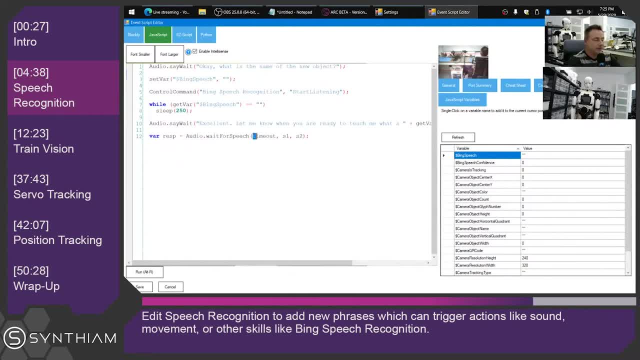 for speech And the timeout is in seconds. So we'll wait for 60 seconds and we'll say, you know, okay or cancel. And now, if the response doesn't equal okay, then what we're going to do is we're going to speak and say: 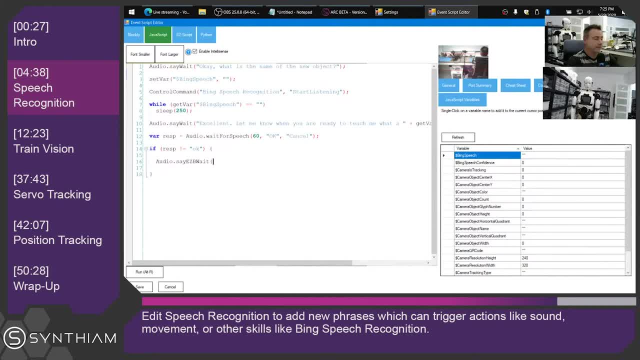 and again we can wait and say, um, okay, I will not learn the and we'll put the variable in here, because we we have the variable. We might as well use it, have a lot of fun with it, And then we'll return from the whole script. So return. you can also use a command called halt. 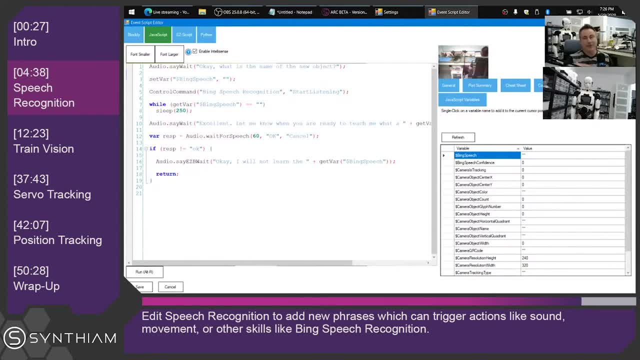 which will exit the script and stop it. But return just means return from the main function, right? So the reason why I put this in lowercase, as well, as you should know, is: uh, wait for speech, We'll always return. whatever the phrase is, It'll always return it as a lower case. 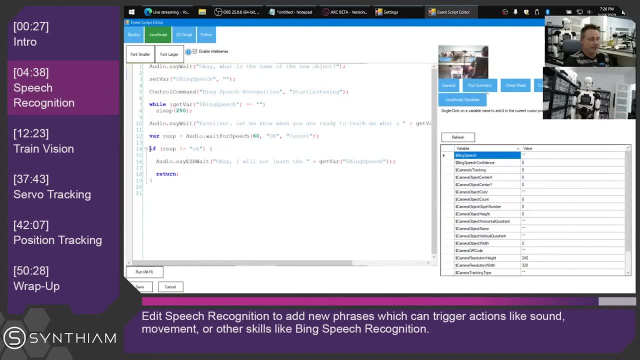 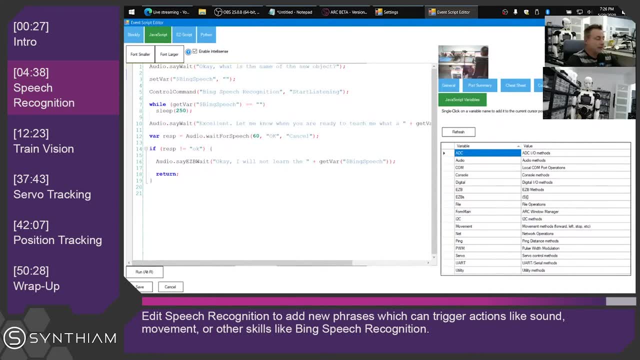 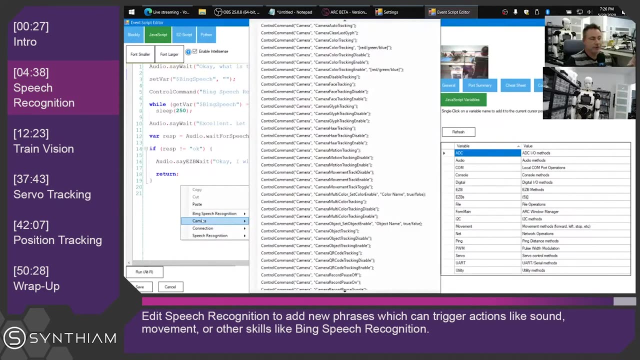 And you'll be able to see that when you look in the variable manager um later, after it's ran, you'll be able to see that the response object is contains lower lowercase. Okay, So now that we have that um, we want to make sure that the camera is not currently tracking anything at. 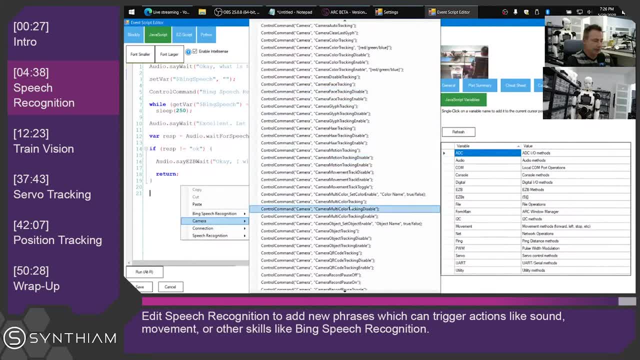 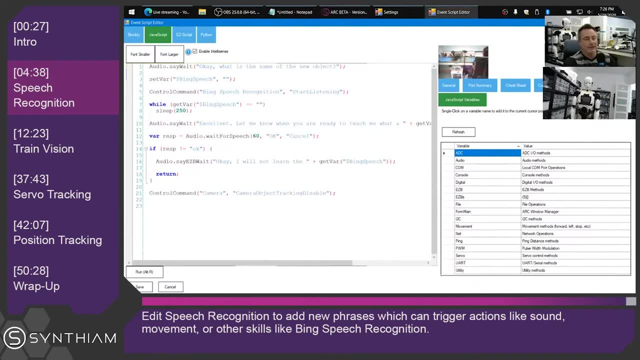 all. So we want to disable, um, object tracking. So let's go to object tracking and we'll say disable, And because we don't want to track, we don't want it to learn anything while we're training it right at the same time, because that would get really confused. 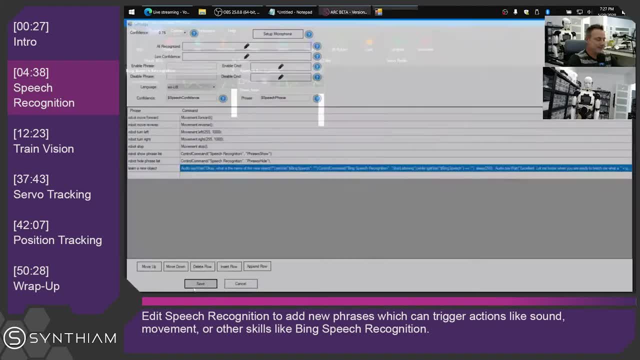 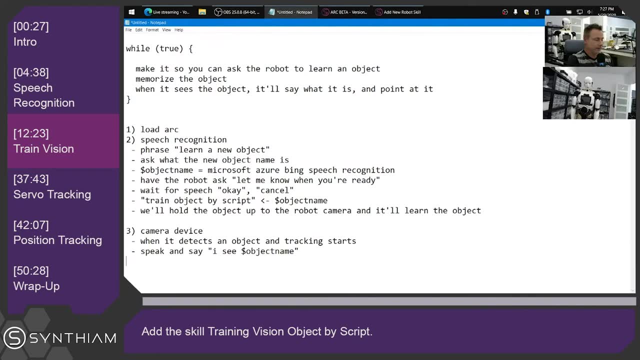 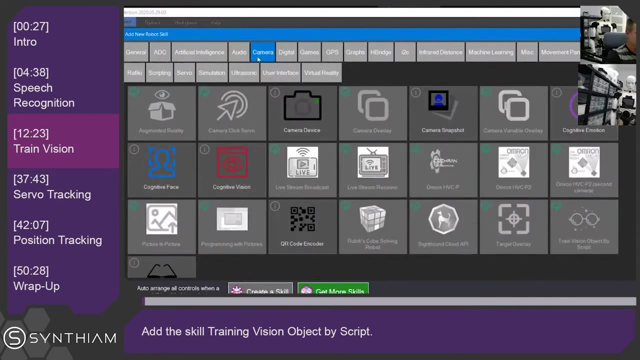 And now we want to save this because we're missing a control, and the control that we're missing- And I mentioned in our in here- is something called train object by script. So this skill, this control skill, here is train object by script, right here. 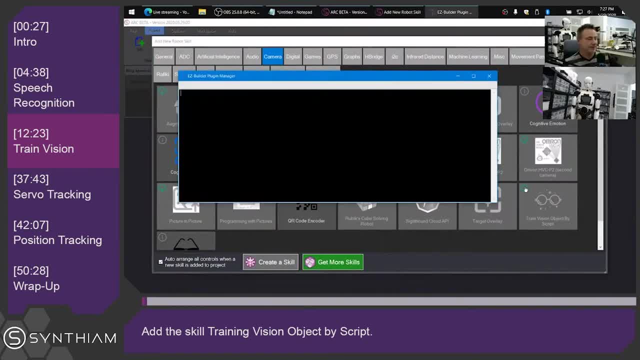 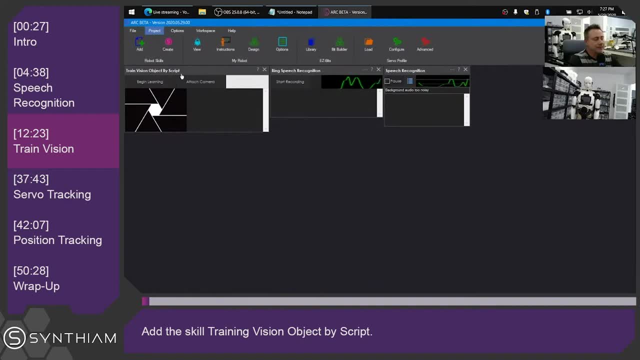 train vision object by script. So we'll click on this and download it, install it. Okay, There we go. So what this will do is this will um, we'll connect to the camera and it'll run through the whole training process. 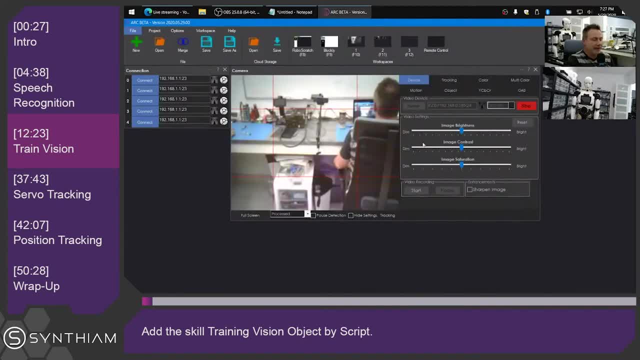 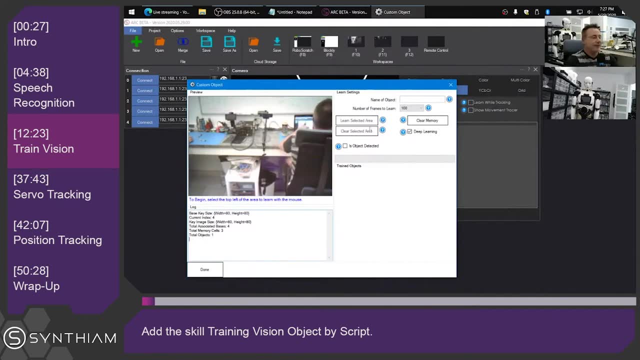 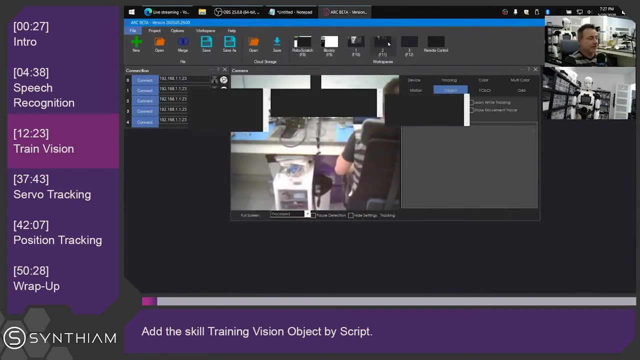 So, as you might be familiar with already, when you're using the camera, you have the ability to go to object tracking and, say, train a new object, And you can go through this whole process. This process is- uh is- a manual normally, So this, this robot skill, will do it for us. 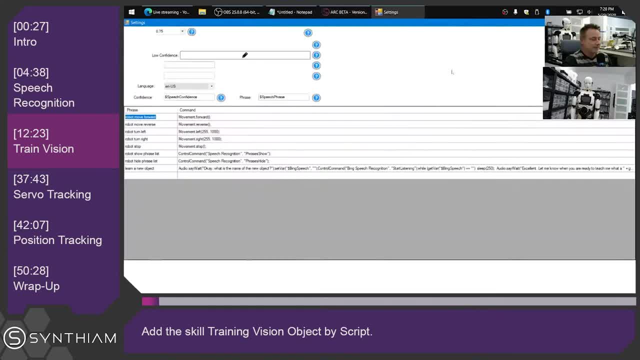 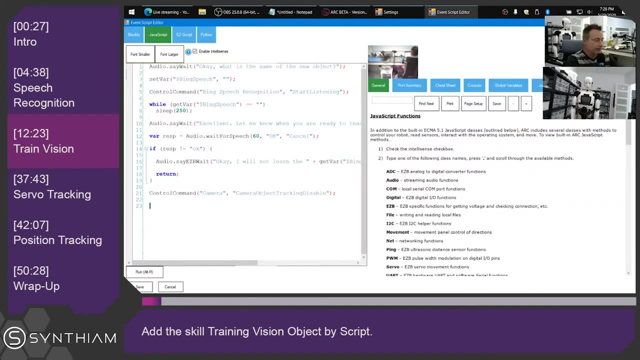 essentially: Um. so let's go back into our code. and now we want to tell it to start training. So we go train by script and we say learn, and it wants the object name as a parameter. So the object name will give it, as you might have guessed. 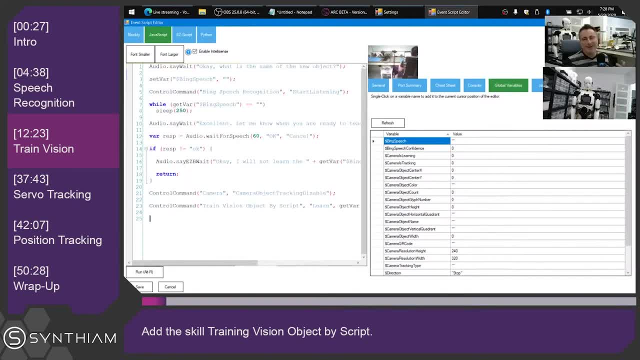 is the being speed recognition. So that's it's going to learn the thing that we told it already And now we want to like wait until it's completed learning. So let's do a while loop And if we look through this list, um, there should be under global variables here. 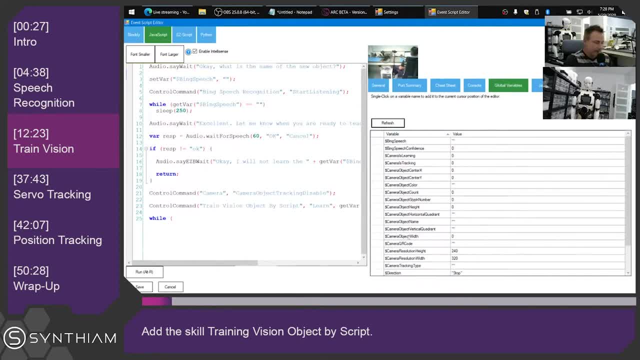 something called is learning. There it is, Camera is learning Boom, So we want to uh loop forever while it is learning. We probably want to put a short sleep in here too, of like maybe one second is good. So that way it gives it enough time to boot up, So it starts learning. 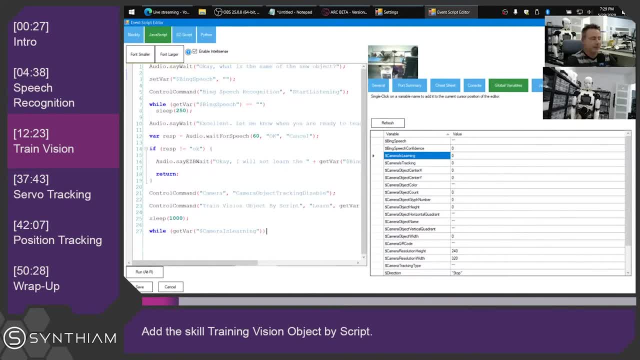 and then the variable will be set. The variable will be set And then, uh, we'll just sleep through this And it's nice, if you're ever doing a while loop, let's close like this, like a really tight. it's called a tight loop. 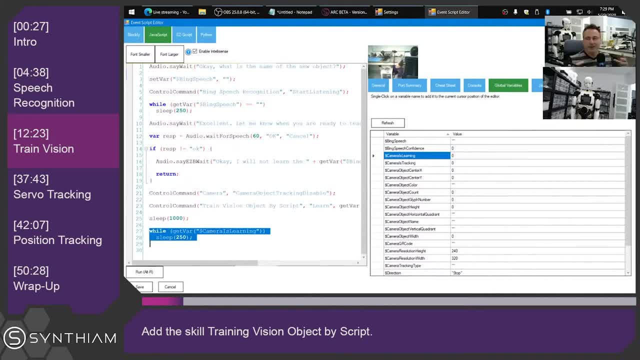 Um, it's nice to put a sleep in there because this is multi-threaded, right, All of arc. And if you're just generally doing programming at all, I shouldn't, right. If you're looping for something real quick, just know you're gonna use up all the CPU. So by putting a sleep in there, 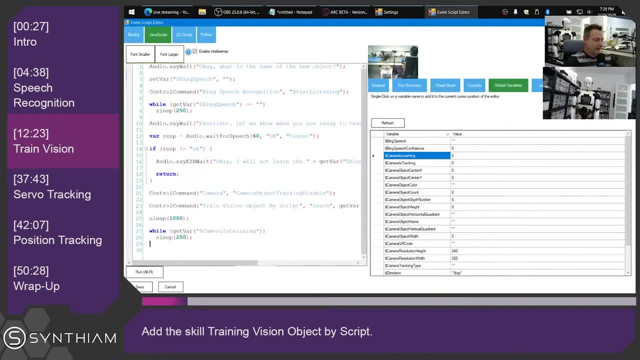 you're allowing other threads to have access to things, And what we'll do is: this is going to loop forever while it's learning And then, once it's done, we'll have the robot speak again and say: great, I know what a- and I'll put that variable in- is. 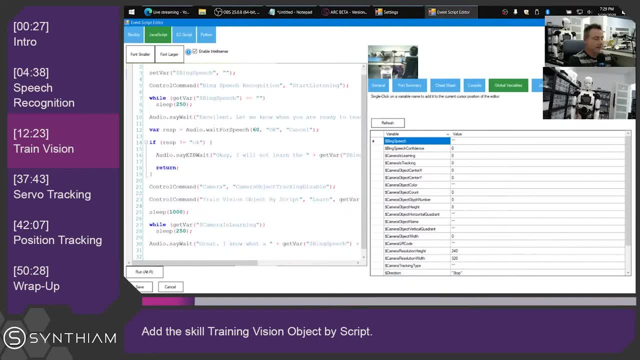 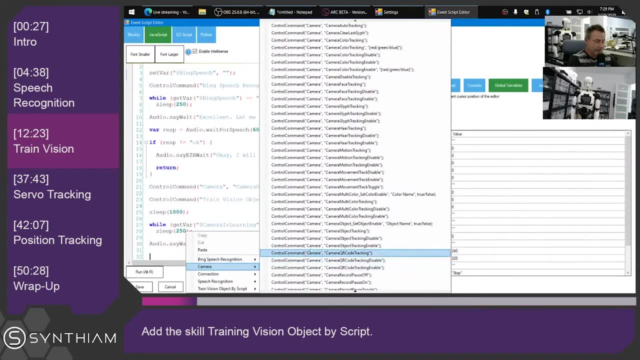 And then we can turn on object tracking now, because now we've learned everything and we'll go back into our here and we'll go object tracking. And then we can turn on object tracking now, because now we've learned everything and we'll go back into our here and we'll go object tracking. 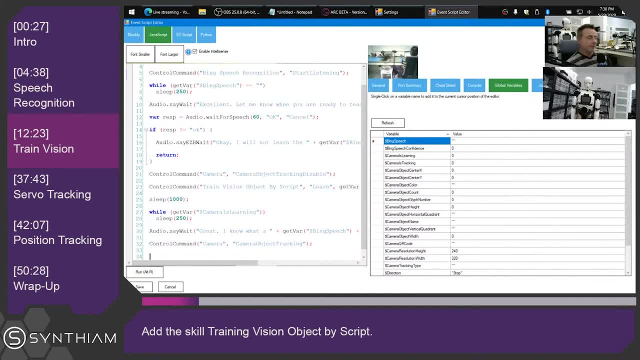 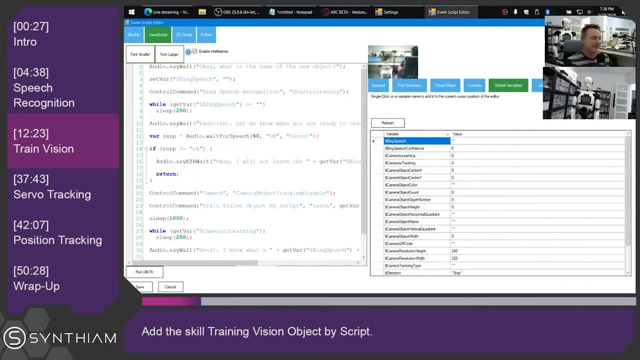 And it's turned back on. So I mean in my head it should work, but we'll find out when we actually push the run button and see. So let's start by testing it. Um, let's just do a full on test. Let's just do this. Here we go. 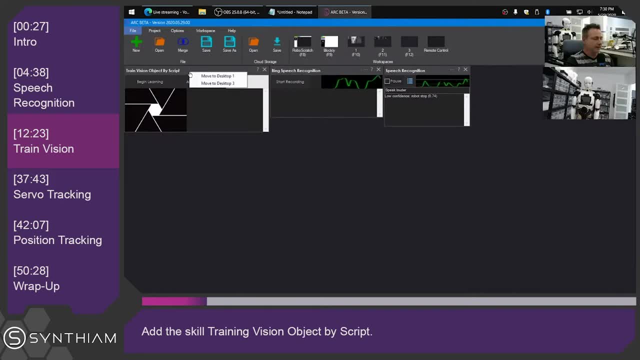 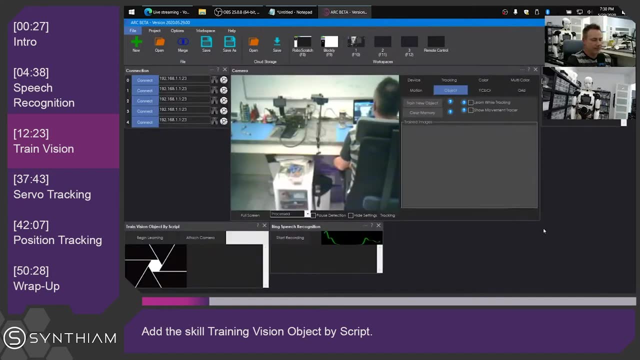 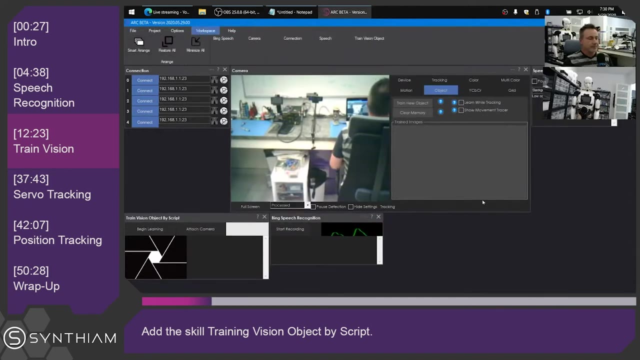 Now I think I'm gonna need the these all actually on the main desktop only because we need to see in the camera and we'll have to make this window a little bit smaller. sort, there we go, and i'll put the speed recognition down here so you can see it. 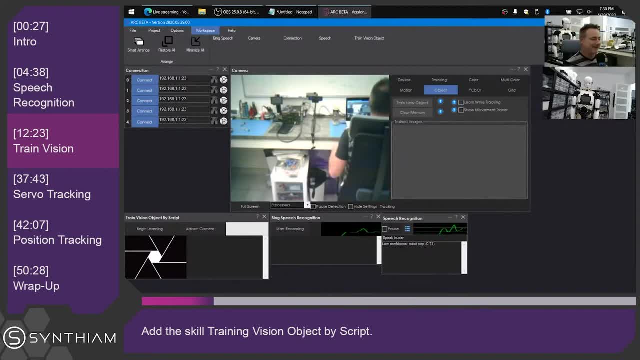 there just because because my head's in the way in the little window, all right, and we'll turn tracking on here or we'll keep it on object. we can see the objects grow as we add them, if this works, all right. so let's do our very first test. here we go: learn a new object. 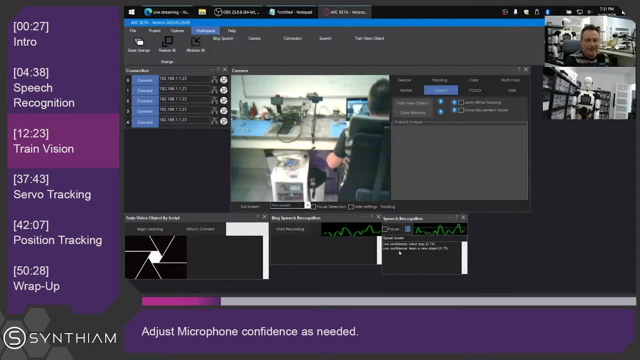 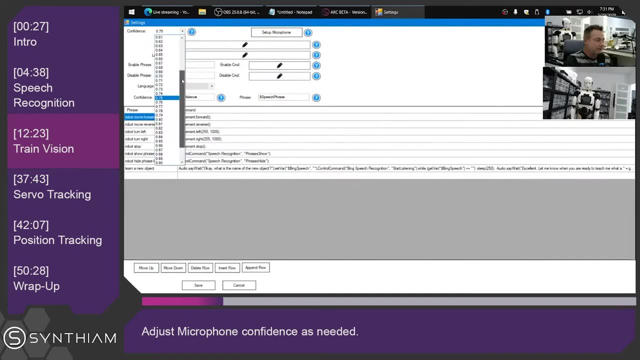 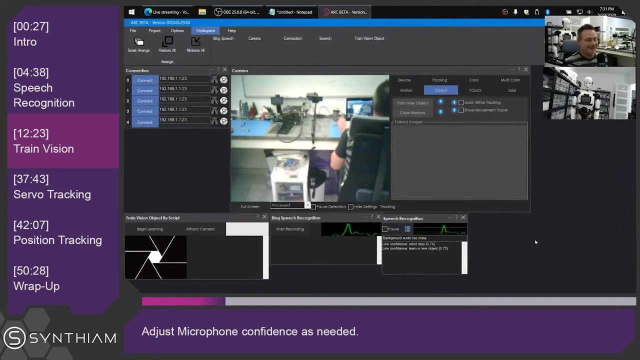 okay. so it did detect that. i said it. but it said low confidence. it said it was 75. so this microphone is not the greatest. let's turn down the confidence. let's make it, um, you know, 60 is probably fine. it's really low, though i wouldn't suggest that if you're using a good microphone. okay. 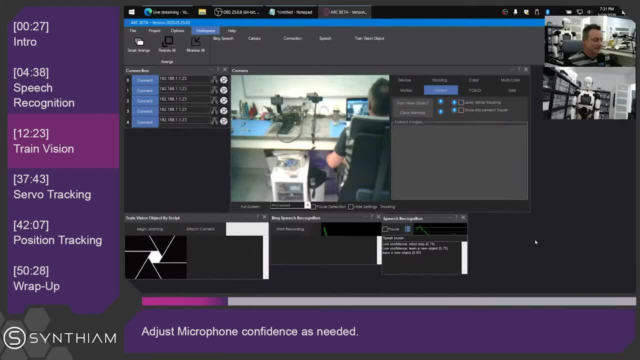 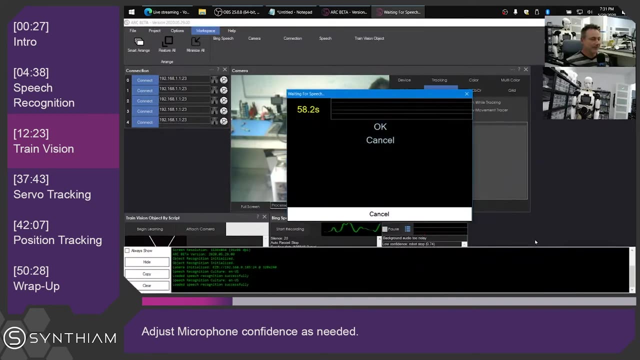 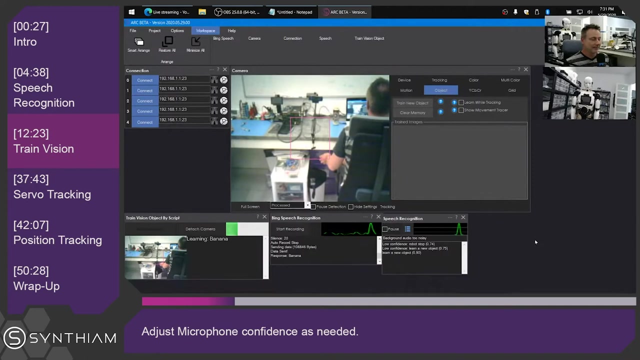 learn a new object. okay, what is the name of the new object? banana. excellent, let me know when you are ready to teach me what a banana is. okay. so it's learning what a banana is just in that middle of the box, so that's not very useful. great, i know what a banana is. okay. it thinks a banana is my arm. 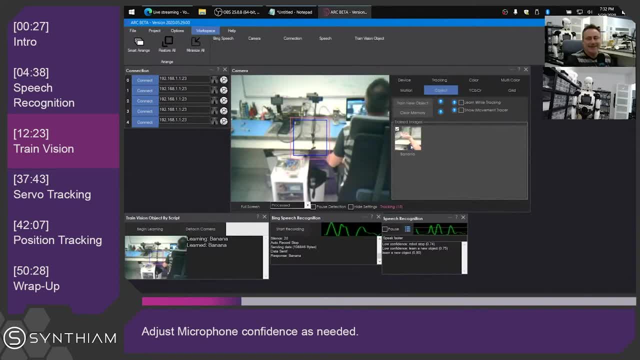 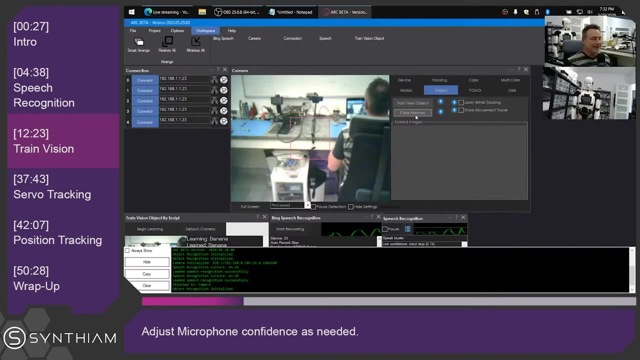 and the desk. so, uh, we can see it here. it actually added it, so it's great. so we can actually clear all the memory that it's learned, because that's unnecessary now, when it detects the object we want the robot to to do something. so let's wait until. 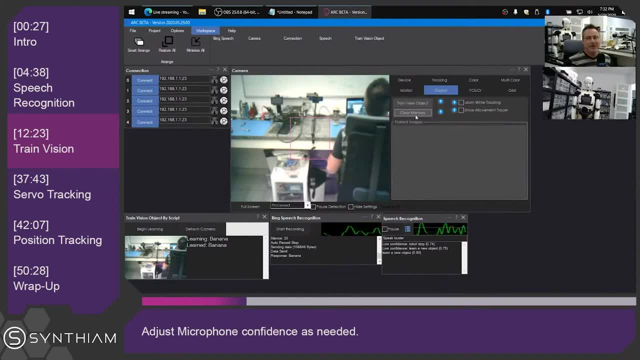 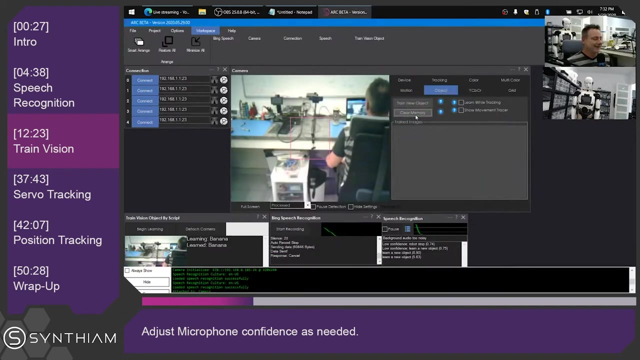 um, we get this on this project onto the end move and then it can actually, um, it can point and speak. So, okay, What is the name of the new object? Cancel, Excellent, Let me know when you are ready to teach me what a cancel is. Cancel, Okay, So that's something to notice, that it. 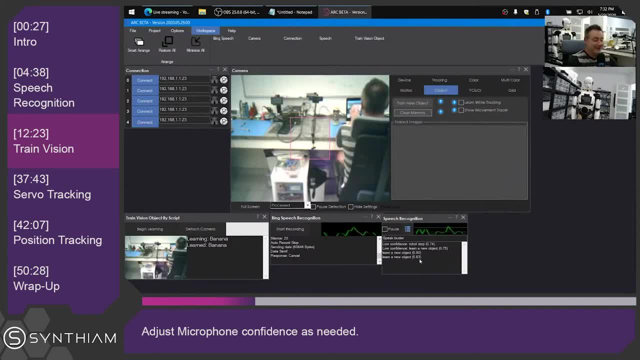 detected what I said. um, because I did actually say the words. you know I don't want to say them now cause it's going to hear me again, but I did say the words. So it wanted to pick up Now I did. 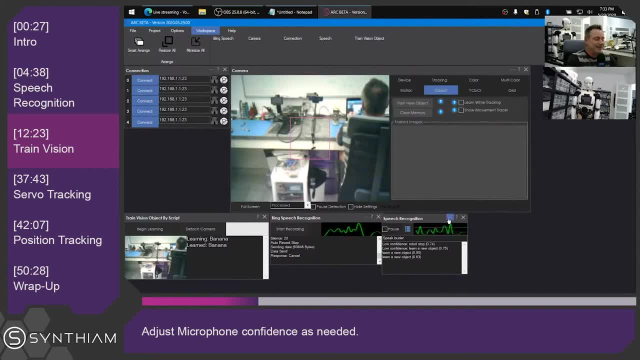 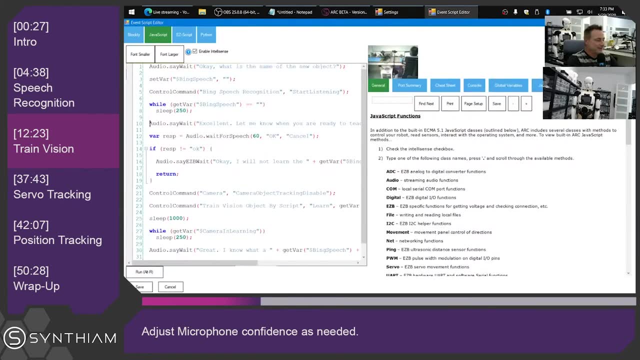 say the word cancel when it said what's the object called. What we can do is we can actually add um some code in here, just like we did up above. that we'll do the same thing. So we can just say if- uh, let's see, wait for it to finish. Okay, Right here We'll just say if the variable 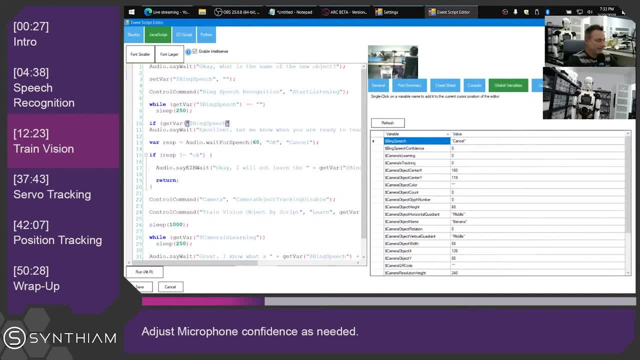 that of being speech recognition, um equals cancel. then we'll just do the same thing here, Uh, with the same thing we did below, as we'll exit. So we'll wait and say canceling and then we'll just return There we go Done. So now we can if we accidentally, uh, if it starts here at 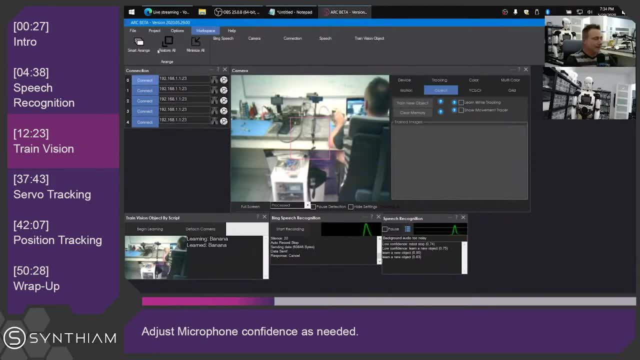 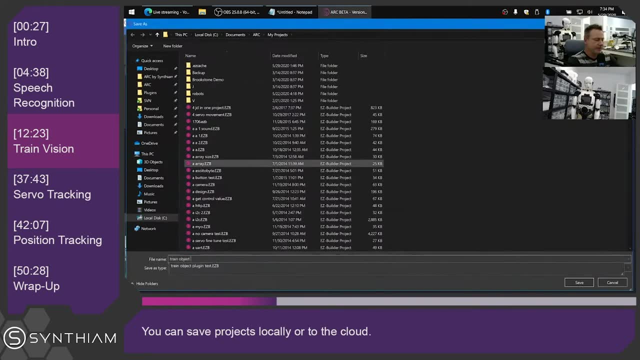 listening to us. we can just say, okay, we're going to do the same thing here, So we can accidentally, or accidentally hears us, We can exit. So let's save this project. and I'm going to save it to my local computer. We'll just call this train object by script And I'm going to save. 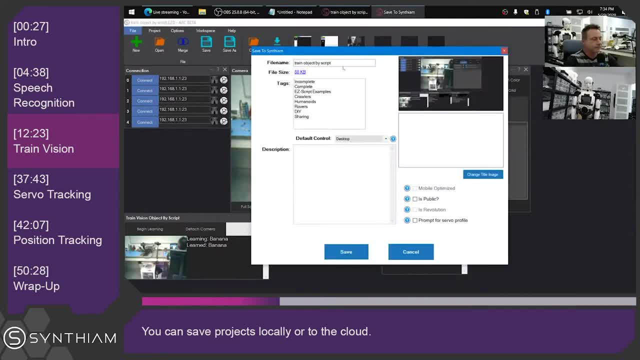 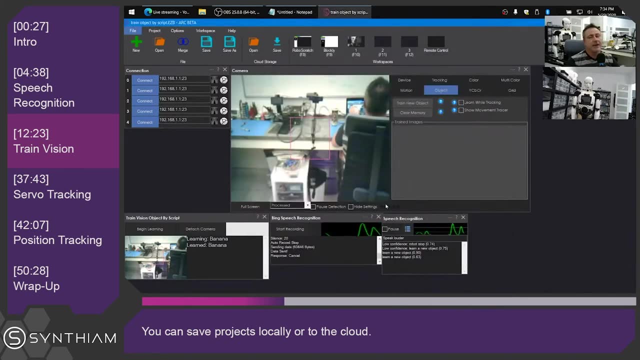 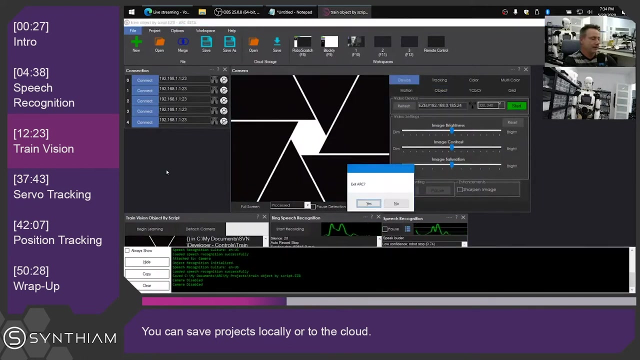 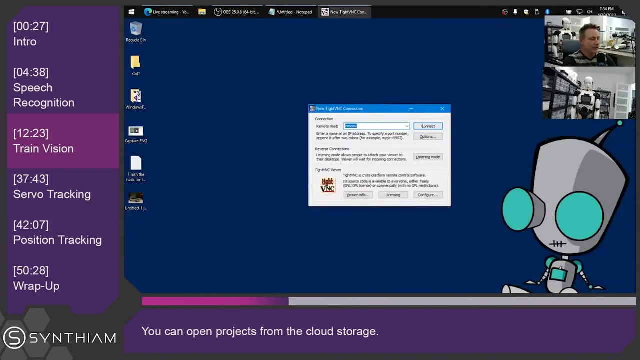 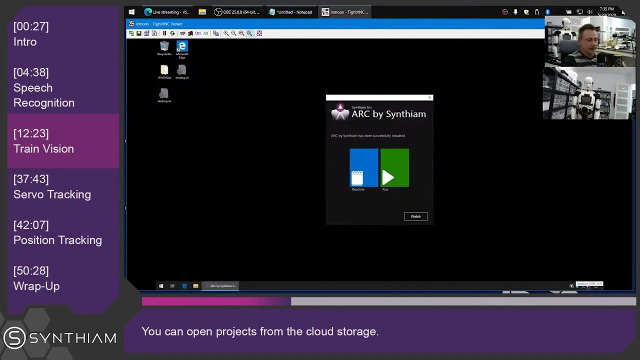 um to the cloud. I'll just say it's incomplete and it's not public, And that's good A description. We'll just- we don't have to put a description Or anything. It's fine, Saved, Nice. So let's close down this project. I don't know why I said that so slow. Let's close down. There we go, Nice. We are ready to rock. Let's make sure that we're running in in a decent, in proper power mode. 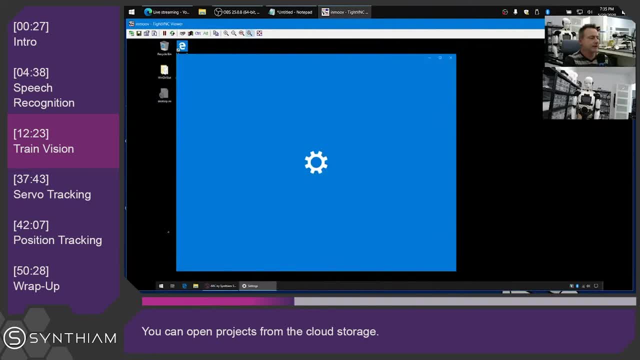 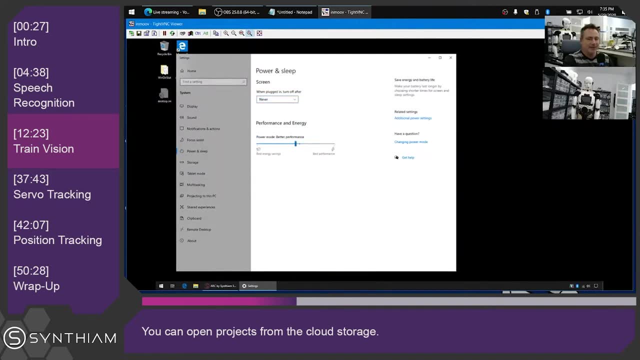 Whenever I've been using computers because Windows has been doing these crazy updates trying to, uh, save the world's energy crisis concerns. So, by default- yeah, this one's already been set, But by default, you'll find that this little under power and sleep performance, energy is in the middle. 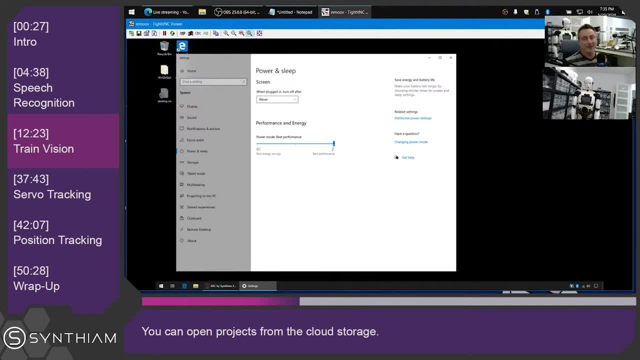 So if you kind of want a computer to work like you know what you paid for, uh, go to power and energy and change it to best performance. You've seen- anyone who's been on my channel before has probably seen me do this often when I'm installing Windows or something. 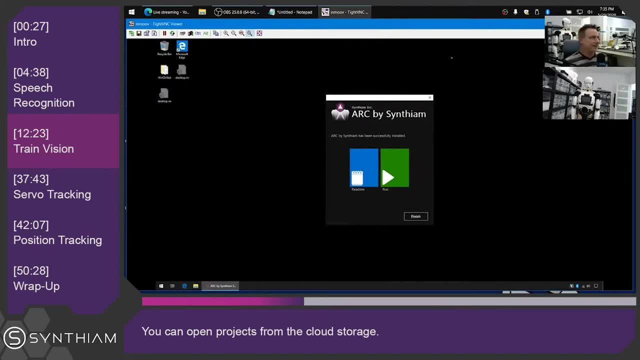 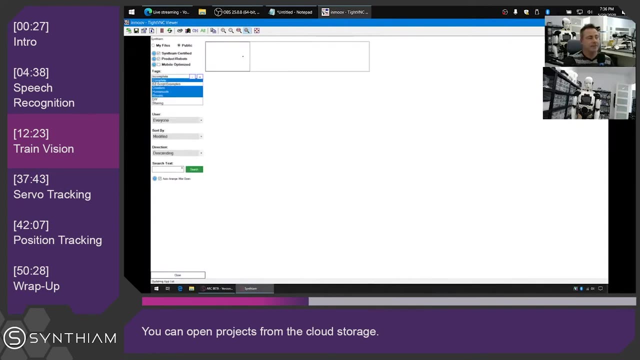 up Windows on SMB, SBCs, single board computer SBCs. Yeah, I have to look at Jeremy, because I get acronyms wrong all the time. Let's go to the cloud storage, because I'm pretty sure that this is logged in as me And we'll go to my files. 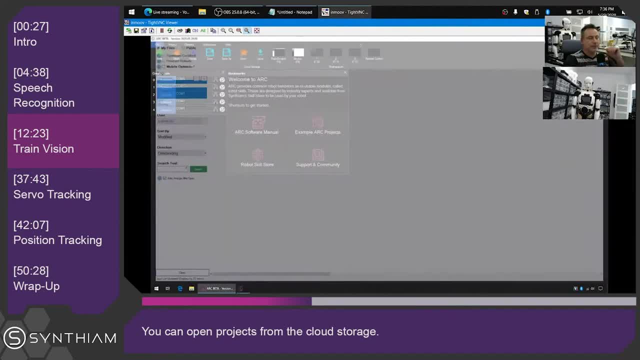 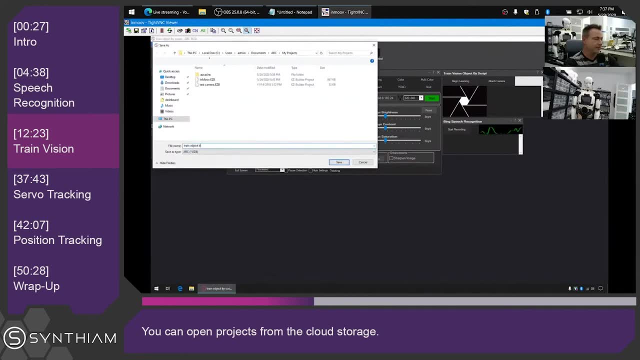 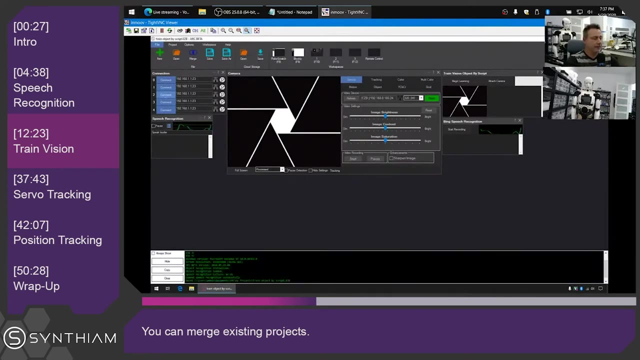 And there it is: Train object by script. That's the one we want. I'm going to save this locally, This project, from the cloud Train object by script, And I think a good thing to start with is: let's merge. Let's merge an existing in move project Because we want the auto position. 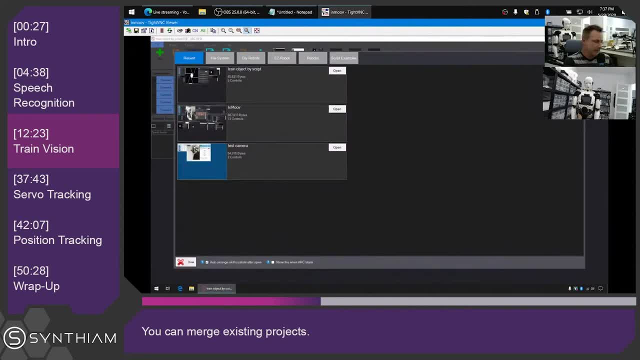 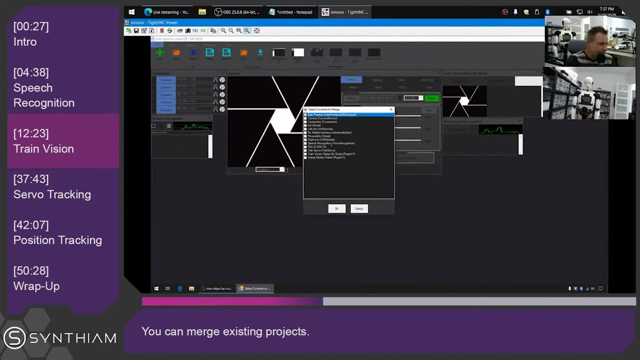 all the movements for the in move. So let's grab the in move project that we already have And we'll look through the list here. We have a lot of things that we want to do. We have auto position- We want that. The camera: we don't care about. 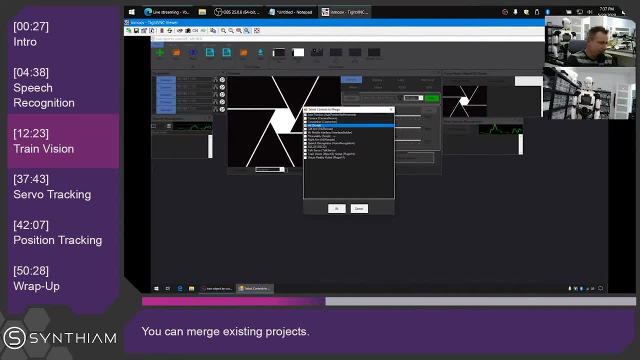 Because we already have one Initialization script. We should probably grab that. I'm not sure what it does. Mobile interface: we don't need- Oh, we need- the SSC32 thing, Because that's an expansion board. I think this is running on an easy robot, easy BV4.. 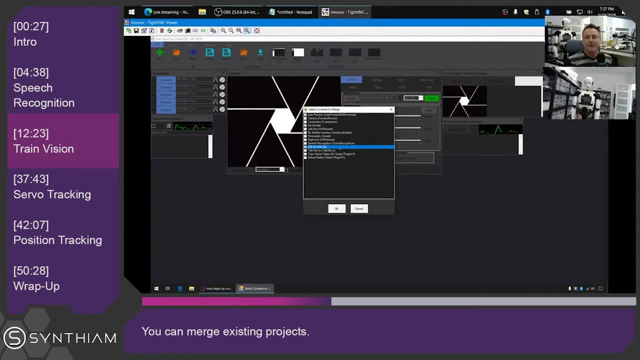 But it only has like 25 digital ports for servos and stuff. So the fingers 24?? Oh, 24 digital ports. So the fingers are hooked up to the SSC32.. This in move, by the way, was built by Richard Ryerson. 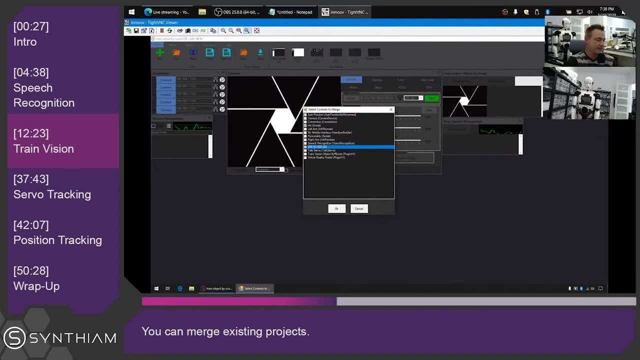 So not us, Not me. I cannot get credit for this thing. This is the one, This is the bartender that pours the wine: Talk servo. Yeah, let's add that Talk servo would be cool, Because then he moves his mouth and speaks the words. 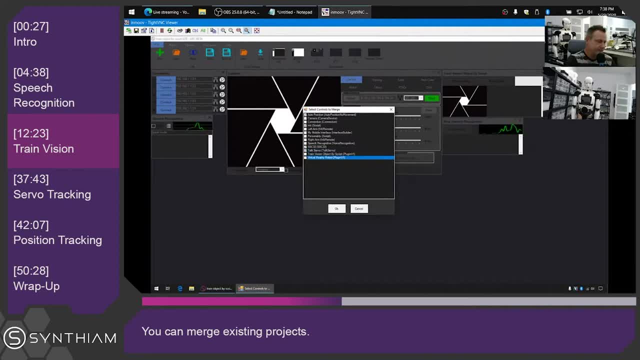 And then train object by script- Oh, there was already one there, But we don't need it. And virtual reality robot: Oh, we don't need either of these. The virtual reality robot is pretty cool, though, Because you can control the robot with your headset. 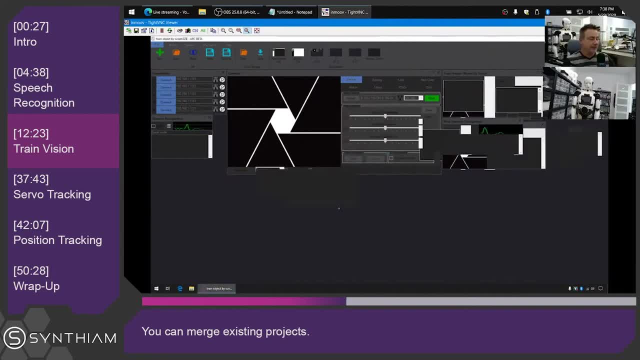 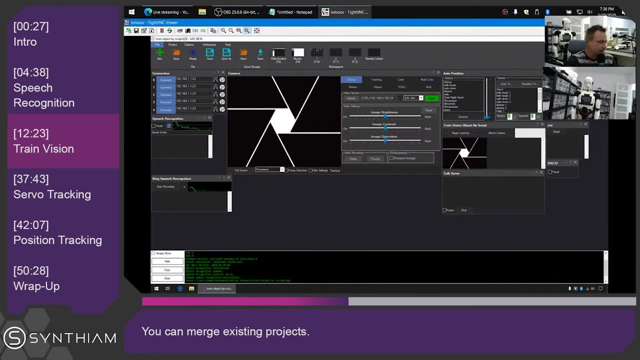 Okay, I digress. Let's click OK And import all these wonderful things, And I'll save this. So now our new project has lots of goodies in it. The camera that we're going to use- There's already a camera. that's a Microsoft cam- in the InMove. 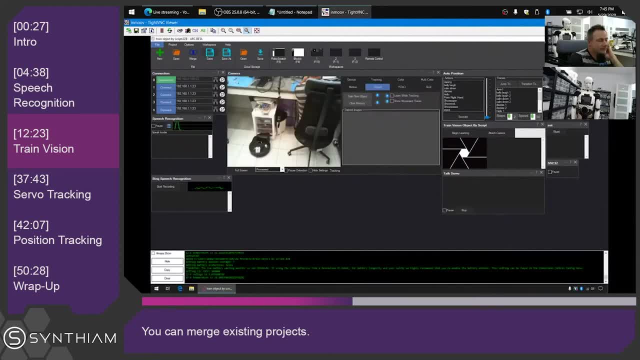 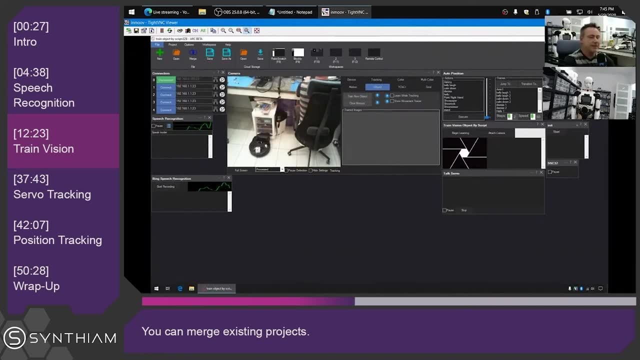 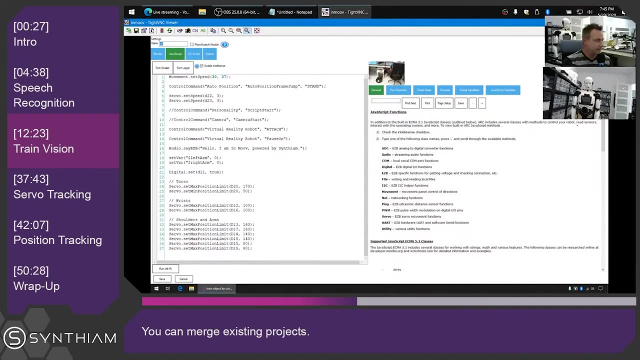 Let's connect to that. There we go, And now there's initialization script. I think this script needs to run. Let's take a look and see what's inside of it. When the InMove loads And this script, what does it do? 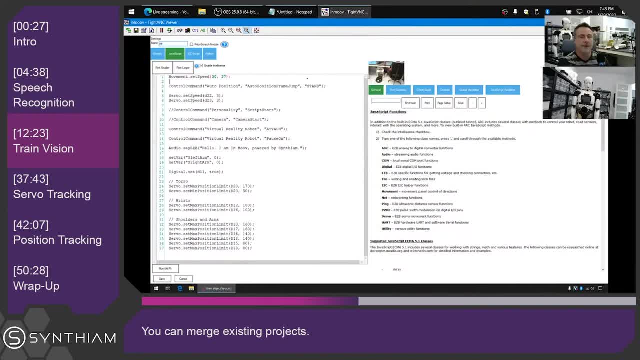 It sets some servo speeds. I think that's for the head: Moves into a position, Sets some more servo speeds. Oh, this is movement set speed. Sorry, This is. This is the very top one. This is actually setting the speed for, like, how fast the robot can move in a direction. 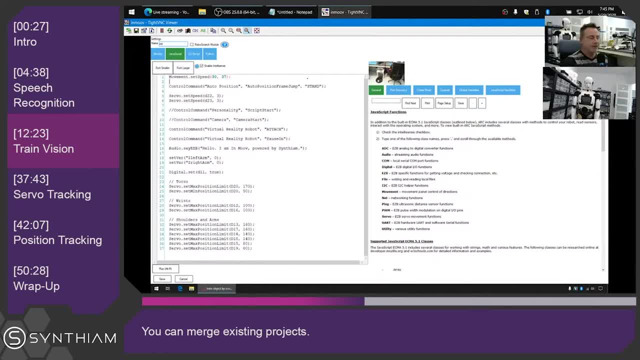 30 is for left wheel, 37 is for the right wheel. I don't know why it's set up that way, But we were playing around with this Virtual reality robot. We can turn that off Unnecessary And it can speak. 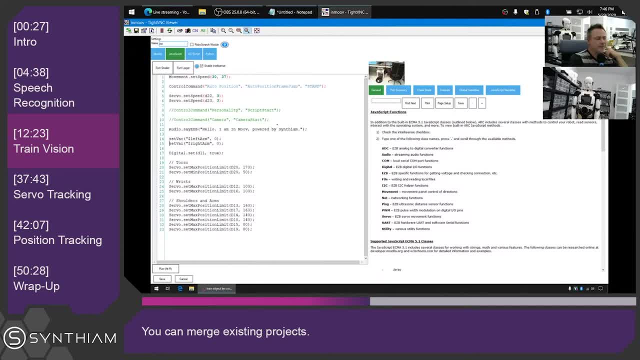 That's cool. Left arm- I think these were set up before these left arm and right arms, because I was using a Wii remote. This digital turn on, I think that turns on the LED that's on the display And then these set the positions, the limit positions, so that the robot can't move too far in a specific direction. 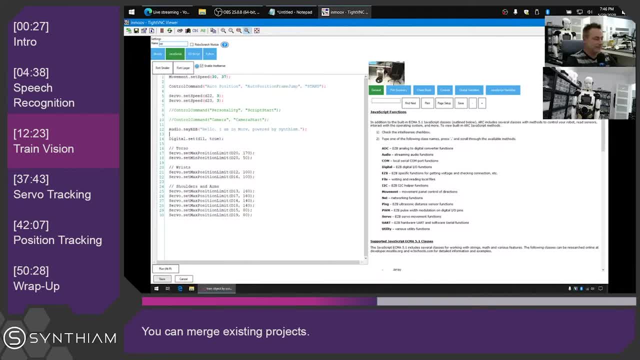 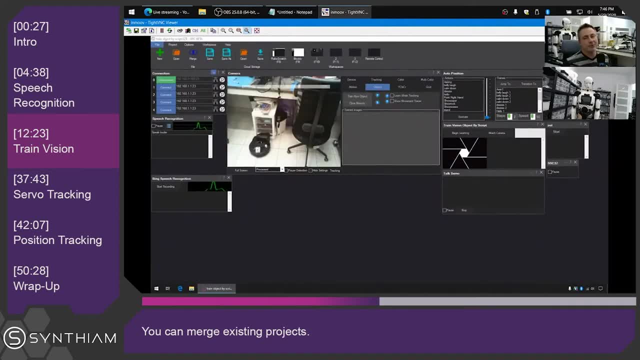 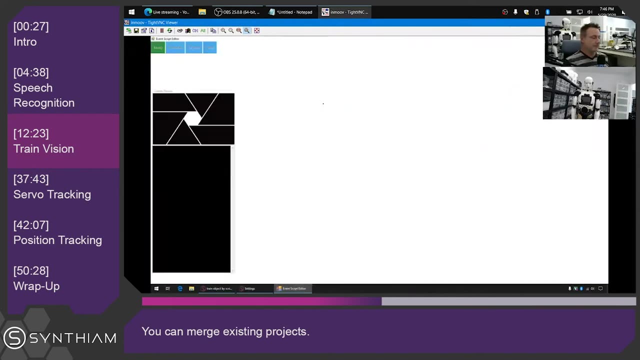 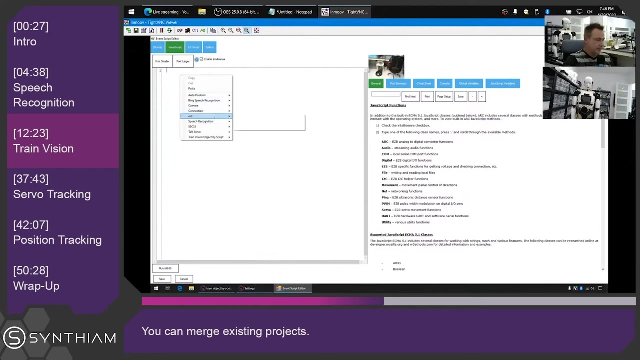 So we're going to keep those there. Obviously those are important. So we'll set the connection control to tell the in it script to run When it's connected. We'll do that in JavaScript here And we'll just say in it script start. 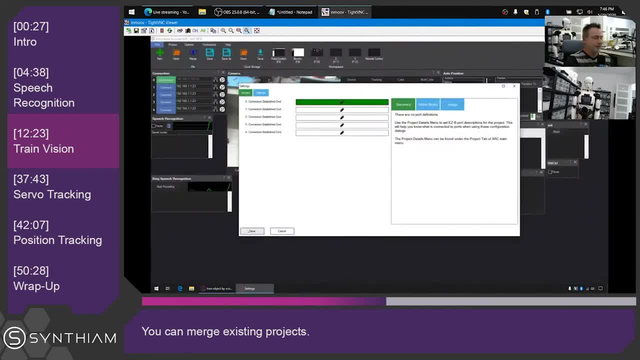 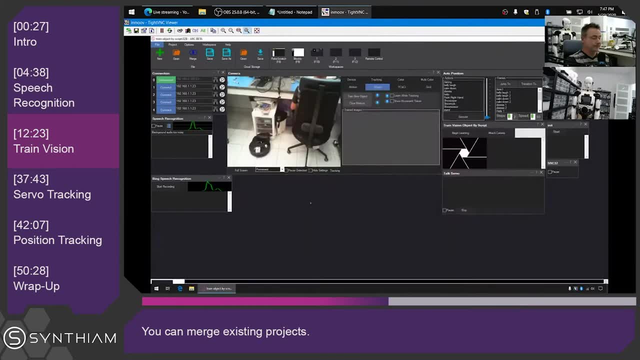 That's it. I really like JavaScript. I use it a lot. It's fast too. Okay, Let's push the start button on the initialization. There we go. So the robot is alive. He is living. now I guess we can just talk to it and do and run our thing. 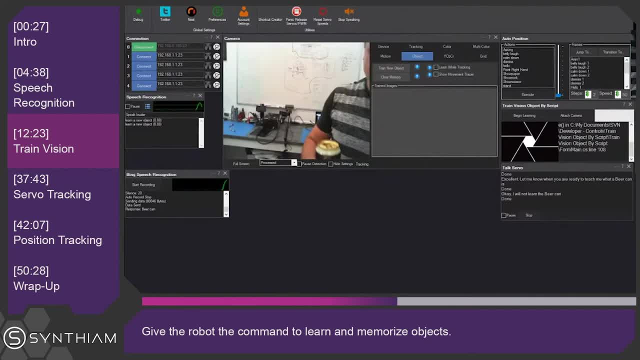 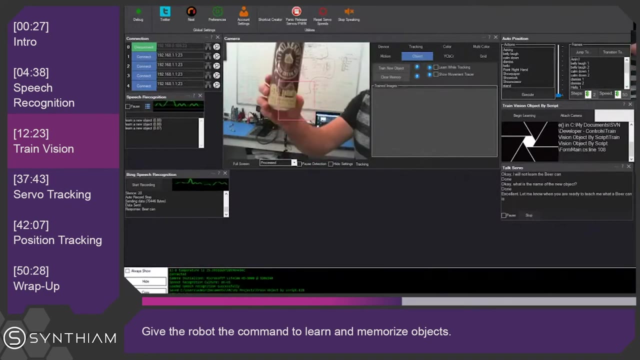 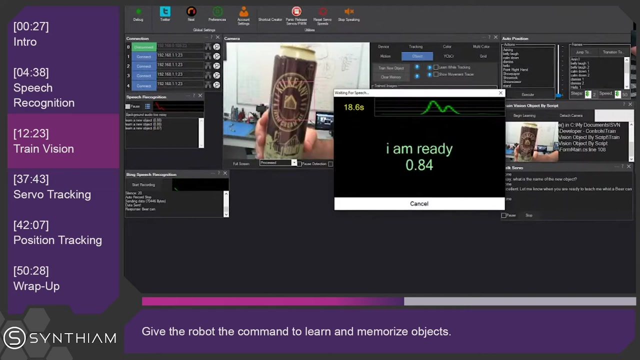 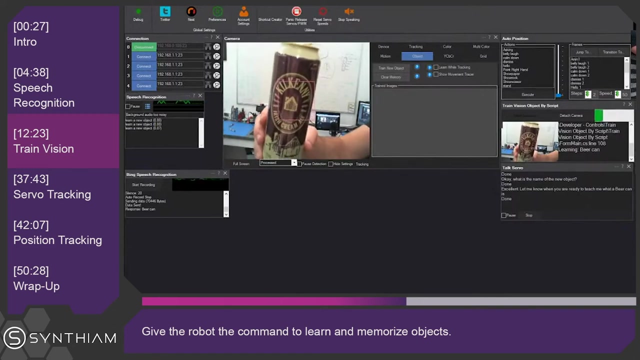 Shall, we try Learn a new object. Okay, What is the name of the new object? Beer can. Excellent, Let me know when you are ready to teach me what a beer can is. I am ready. Okay, so now you can see on the the control that's called train object by script. 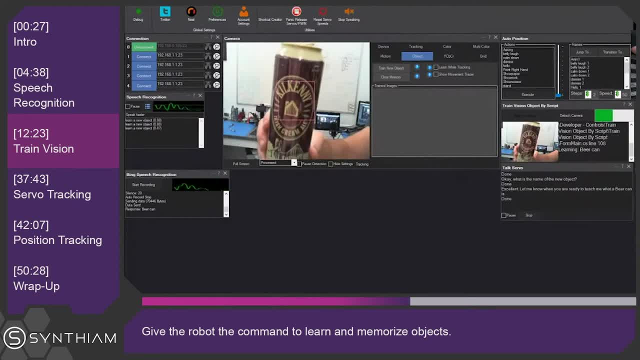 You see, it's got that little progress bar that's moving. That progress bar is showing me how much of the object it's learning. So I want to move the object around in that square on the screen because that's how it's learning the object frame by frame, in different positions. 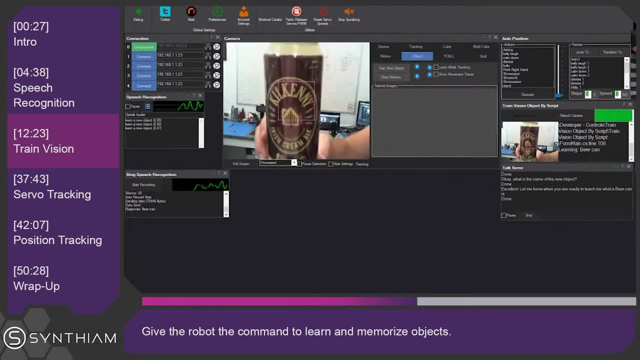 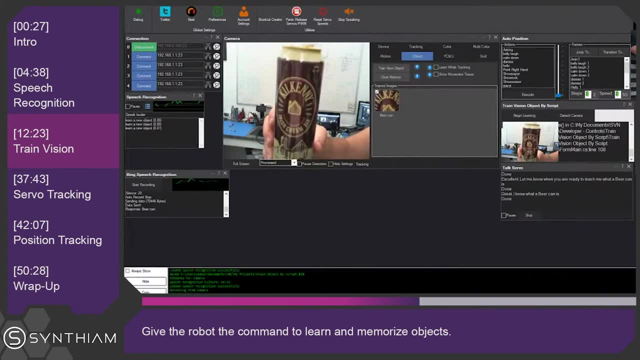 So I want to make sure there's not much background in there either, because the more background that's in there, Great. It's going to see I know what a beer can is. There we go And you can see on the screen that's detected the beer can. 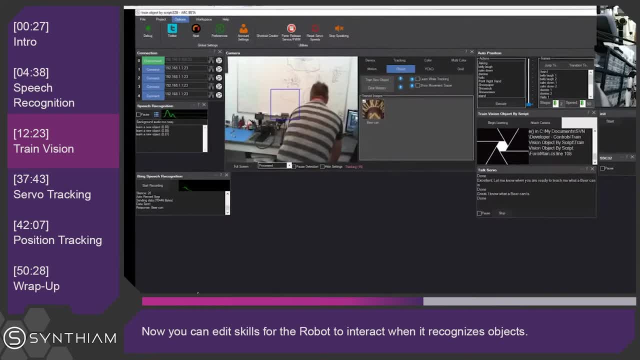 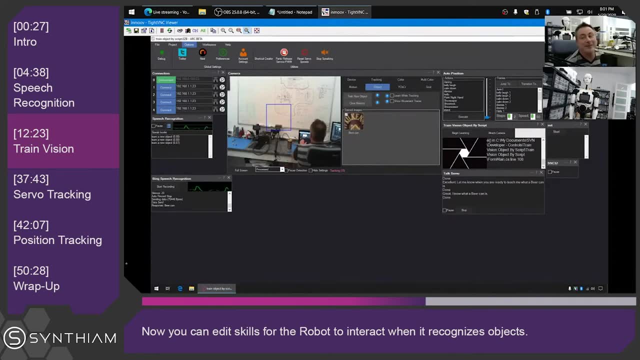 You see, it's put the blue box around it. So we've now taught the robot what a beer can is. Now we can do this for everything, But we want the robot to actually interact with us now, Right, And do something really cool that, when it sees the beer can. 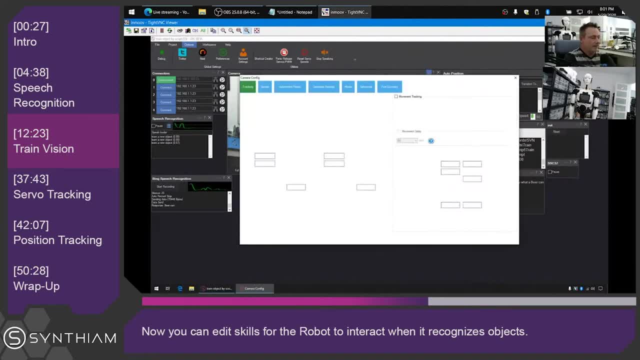 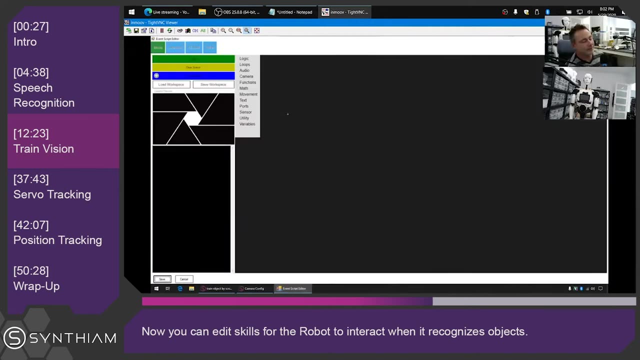 So we're going to go into the camera control And we'll go into a script And we'll go into a script And we'll go into a script And script: start tracking script. So this script will run whenever tracking begins and whenever detects any object at all. 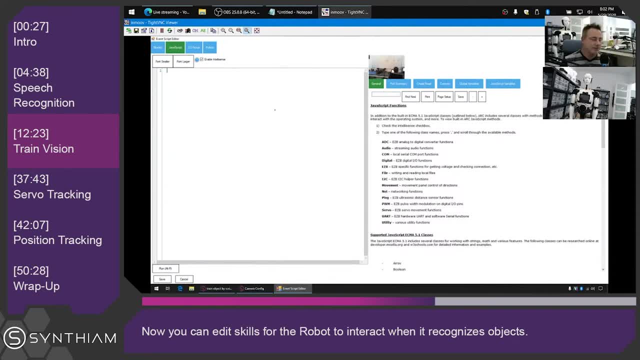 If you have a project that's already doing a lot of other visual tracking stuff, you can always check what type of tracking is being done. So if you look at the global variables here, we're going to see that there's a tracking type in here called object. 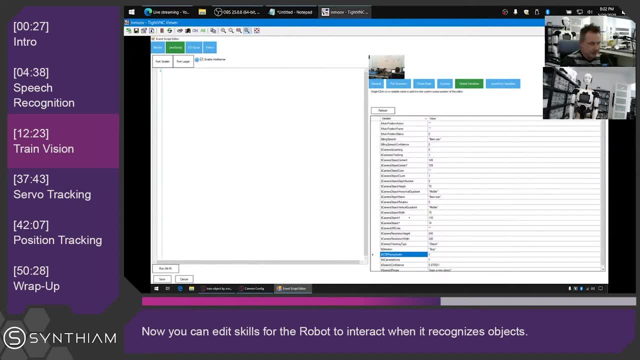 it'll say object type. i think it is tracking type right there. so tracking type is object. it's always a good idea to check to see if the tracking type that you're actually getting is the type that you expect. so we'll say if it's the, you know the tracking type is actually the word. 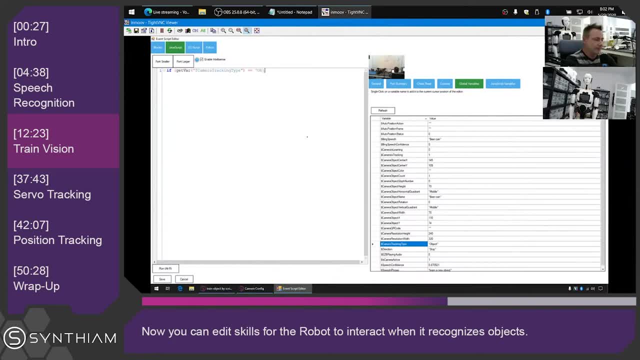 object and case sensitivity is important here. so if it's this, and the reason why we're doing this is because, if you have, if your project for your robot is checking for colors and glyphs and faces and all these other things, you want to isolate what's going to happen for that specific tracking. 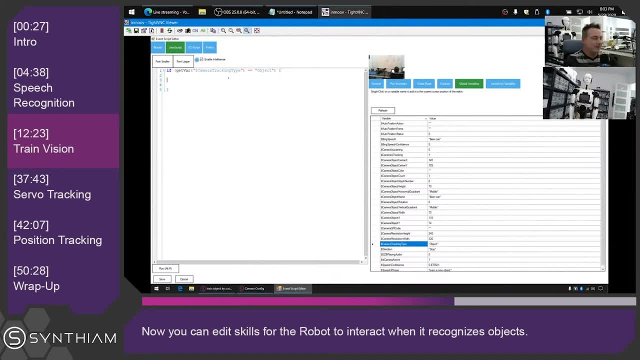 type. in this particular case it's just object. so if it's just the object, we're going to speak and we'll say: out of the microphone i see a, and then we'll put the variable of the object it detected and it's called camera object name, right there. 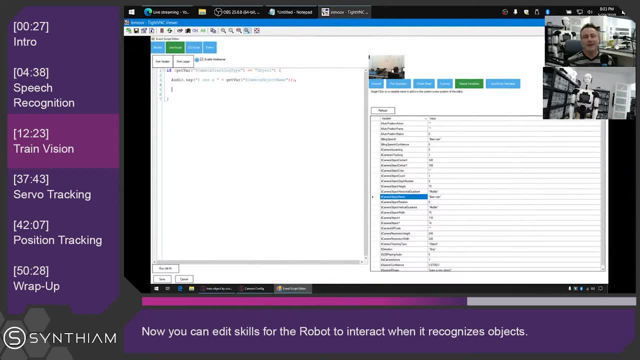 okay, and now we want the robot to do something- um, visual, i guess- like physically. so this robot does have an auto position, which means there's probably a couple different motions that it can move into, and let's take a look and see what motions we have. so i right click in the script. 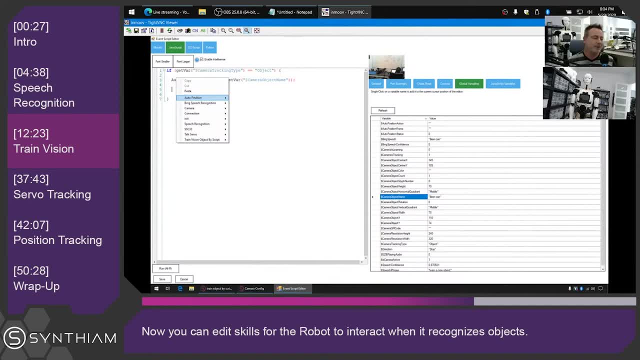 and it queries all of the skills that are added to my project and says what can you do? and they come back and they tell me: so the auto position, it can do um, it can do something called asking. calm down um point with the right hand. let's do that. let's make the robot point actually. let's find out what asking is. what do you think? 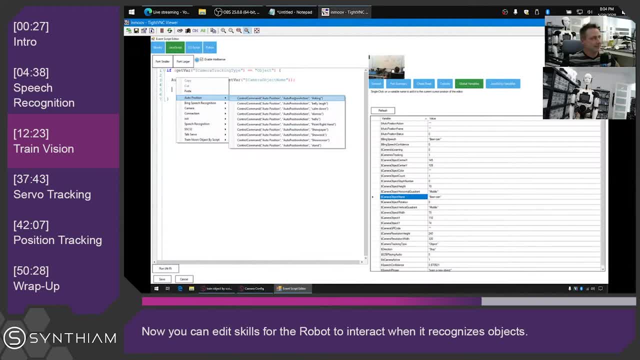 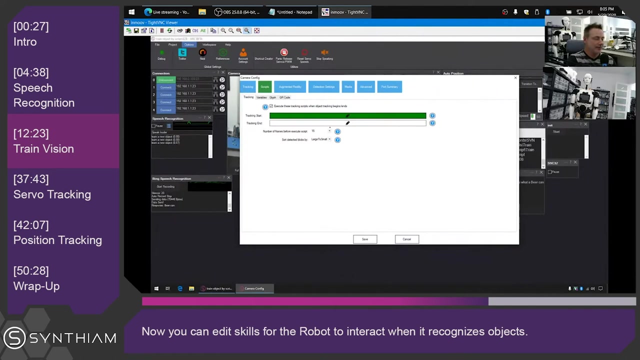 asking is. i'm thinking to myself, i don't know. we have to try that out and see. i don't know if it's gonna work, because asking to me feels like it's not, um, the right thing to use. but there's a whole experiment anyway. let's see. there we go and now, when the tracking ends, that 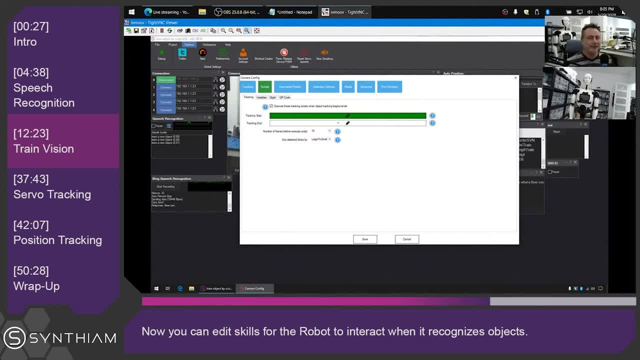 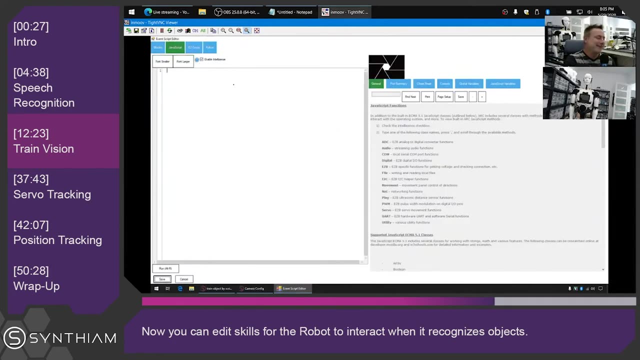 means like you've taken the object away from it and it no longer can see it anymore. we're going to put a script in there too. we're going to make the robot um go back into the standing position rather than you know whatever the asking position is, so you might already have code in here. 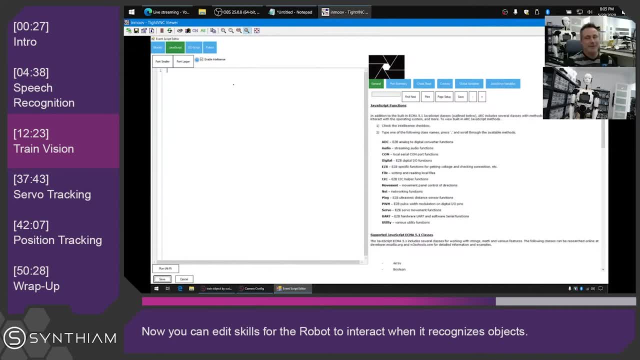 again. you want to check what kind of object track object type was the last detected, so that the same, the same uh thing would apply when the object track type goes away. if we write our if condition and take a look at our variables, we'll see that the object type is is still there. so object type. 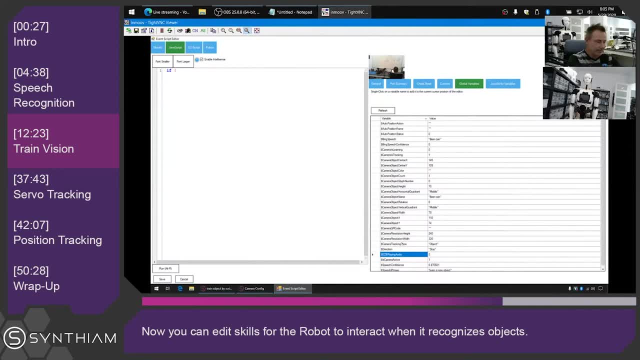 or tracking type, sorry, not object type. tracking type equals object. and again i should add, if you're just, you know this is, this is a project that you're just working on. this is the only thing you're doing. you don't actually have to type these commands in at all. 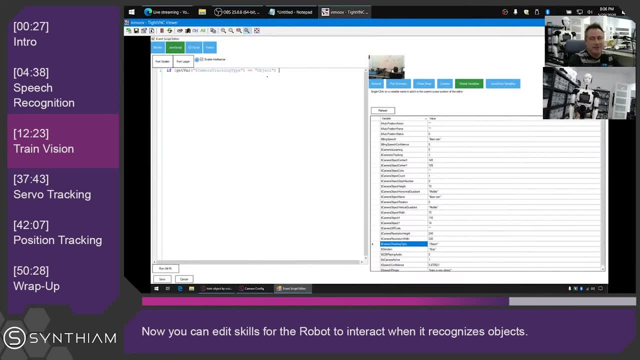 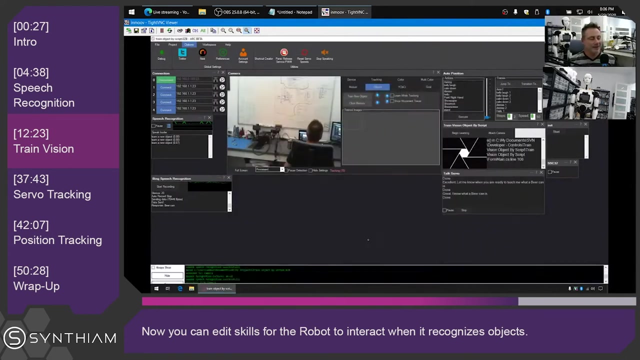 these if conditions. you can leave the if conditions out, because you might just be using this with object and that's it. and now let's make the robot go into the standing position: stand rows. we have like this and we'll save this there. i will save this. 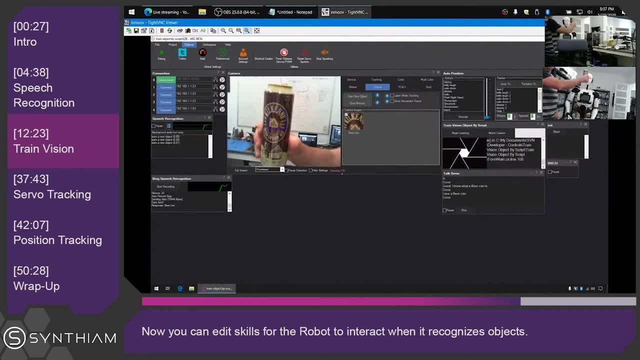 oh, there, it's got it. i see a beer can and he's got his hand on his hip and then now i take the object away and you can see it's counting down here of how many frames we've got to get to. there's two of them here so you can see the name here as well, so you can even put up and save number for like an object in there. 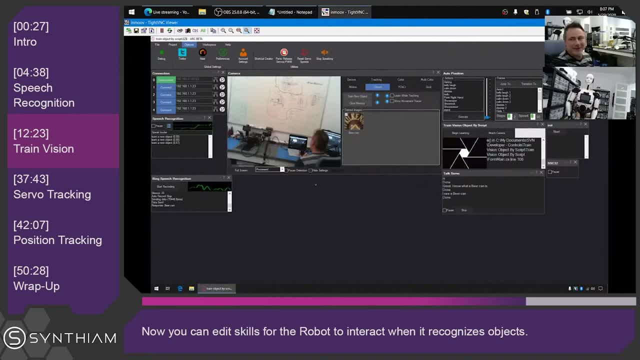 frames, and now it's gone away, and then the robot's going to go back into its original position. so that's cool, so we can teach it something else. now i have a latte panda box. jeremy's offering things that aren't going to work with object training. 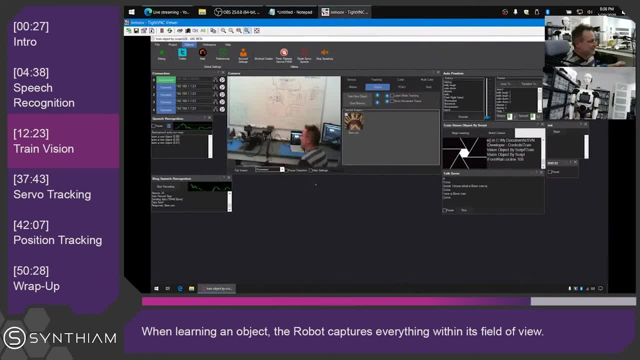 let me show you what jeremy was offering. grab me the pair of pliers or a stapler. it's not about flat. so what, jeremy? i said, learn this now. the trouble is, we kind of can, but you have to manipulate your environment, because when you do object training, it doesn't actually see the object. 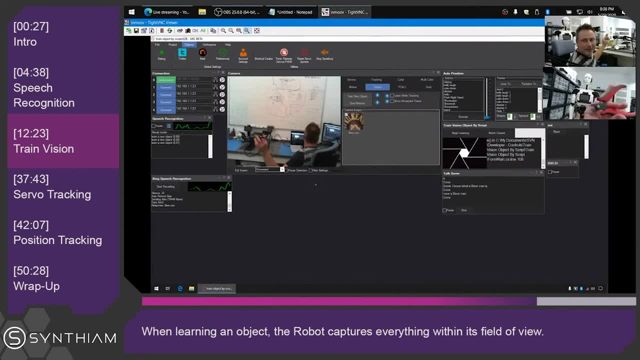 it sees whatever's in the square and if you have something like this and it can see all the background, it's going to learn the background. it doesn't know that this and the background are two different things. right, it doesn't have a clue the difference between this and the door, so it's going. 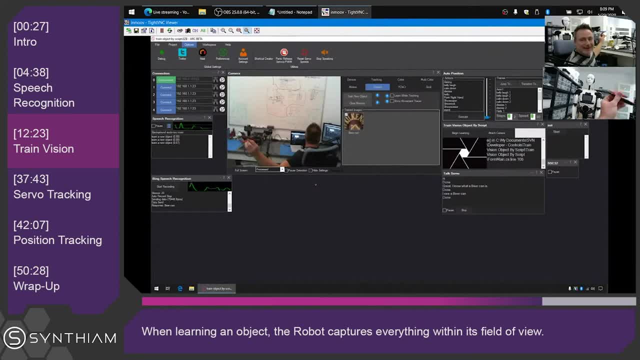 to actually learn the door through the pair of pliers. so you want to put a piece of paper and have a well-lit area without a lot of light, um, without a lot of shadows, because it'll learn the shadows as well. so a very nice white background. 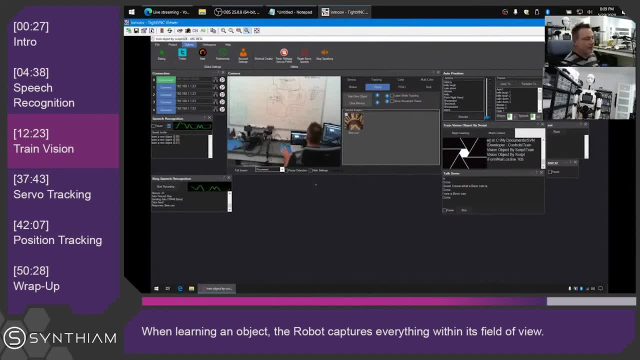 to an object if it's something that you can see through, and then it'll be able to learn it. something else, too, i guess to note too is that when it does learn the object inside of the the code, it actually converts it into a black and white image. so that's something to uh to keep. 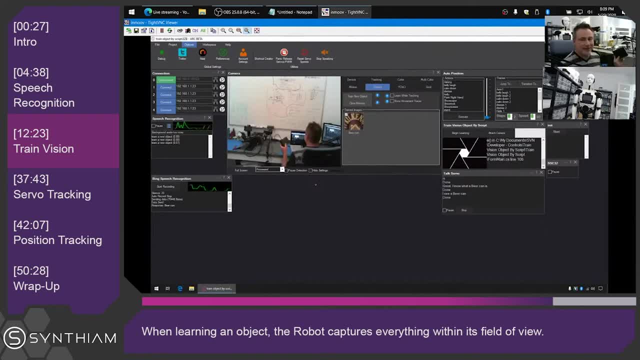 note of. so let's, let's try it again. let's teach it the latte panda box learning new object. okay, what is the name of the new object? latte panda. excellent, let me know when you are ready to teach me what a latte panda is. 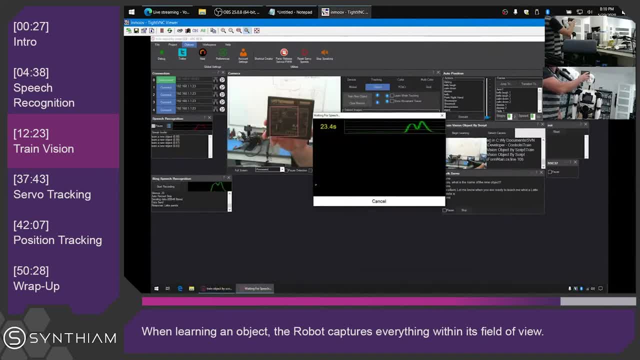 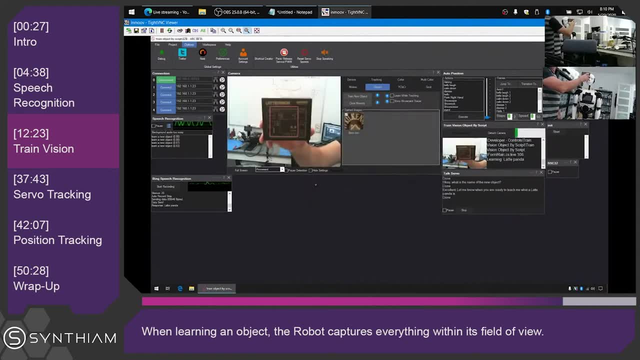 i am ready. great, I know what a Latte Panda is. Okay. So now let's see if it actually does know what a Latte Panda is. So I'll hold the Latte Panda box up. I see a Latte Panda. There we go. 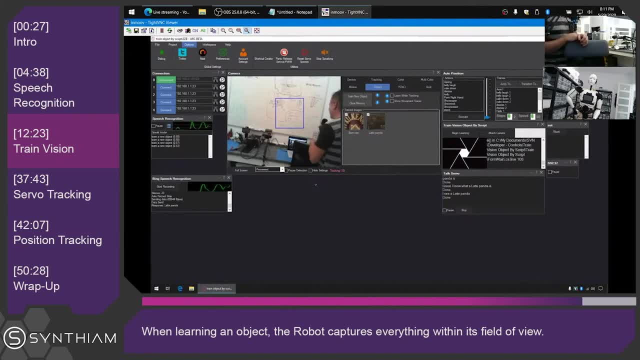 It's perfect. So now it's learned what a Latte Panda is. Okay, so that's a funny position that he goes into here, though I don't know if It just kind of looks like he's got attitude. He's like I know what a Latte Panda box is. 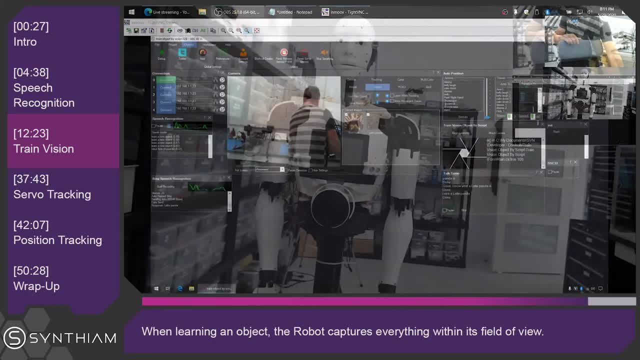 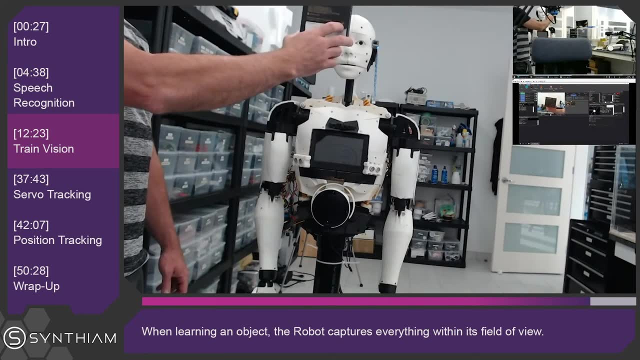 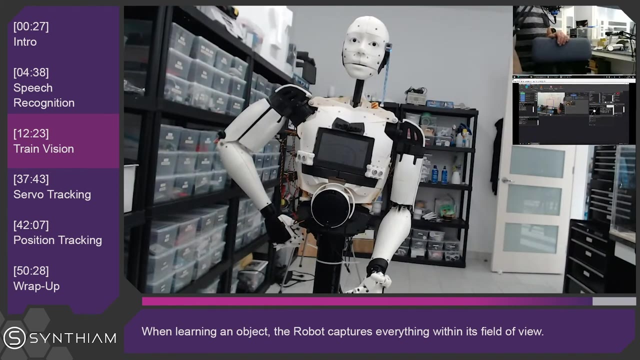 Let's do a close-up so you guys can see what it looks like from here. Okay, so we'll do the Latte Panda box again. I see a Latte Panda. There we go: Learn in my face, Teach in my face. 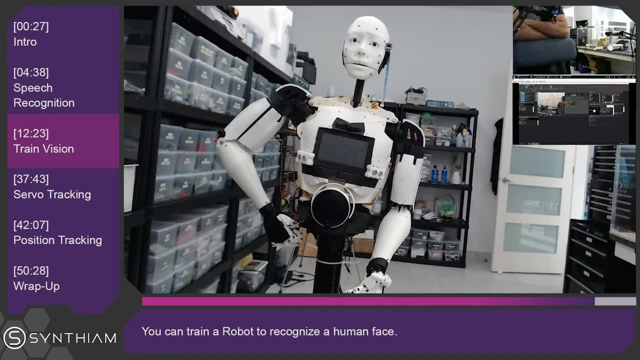 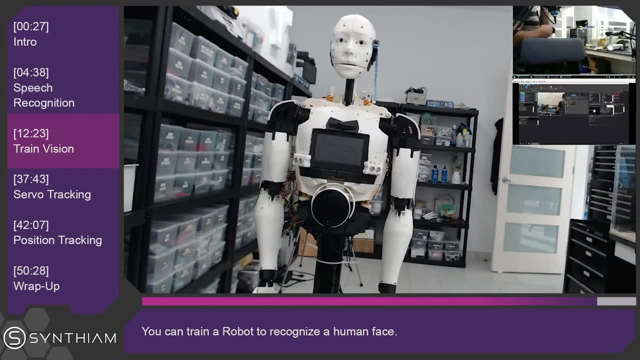 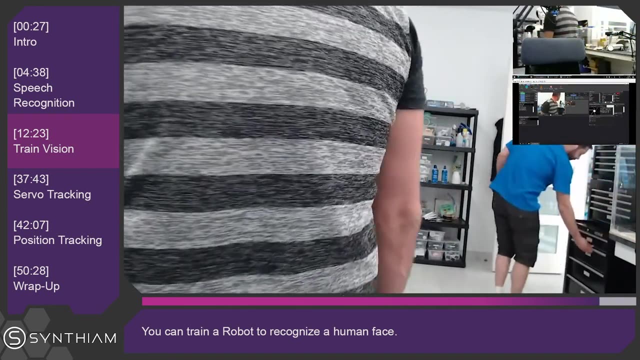 Yeah, we could do that too. Okay, So let's teach the in-move in my face, And let's try teaching in my face. This is going to be interesting. First we'll test. I can't. I'm going to have trouble with this because I can't actually see the screen. 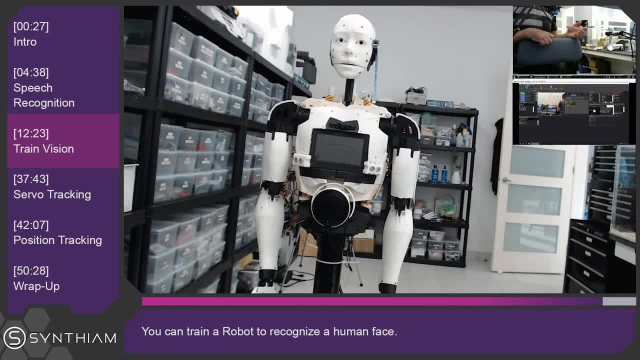 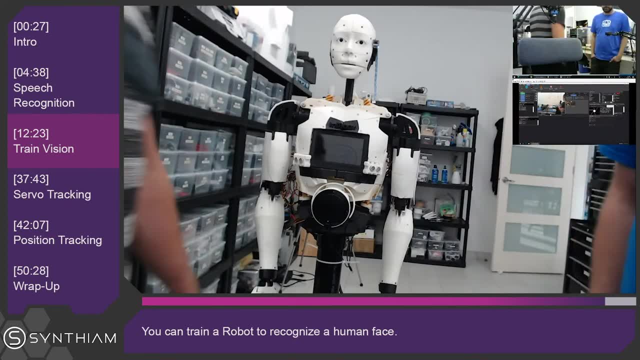 Right, So I don't know where my face is. I can't see the screen. I'm going to have to get Jeremy to help me. Actually, we'll just teach at Jeremy's face How's that? I was trying, but I can't see the screen. 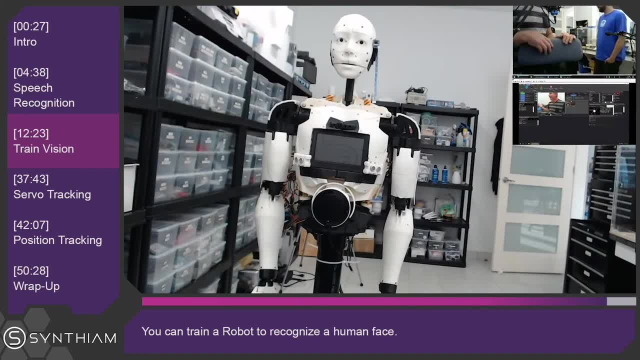 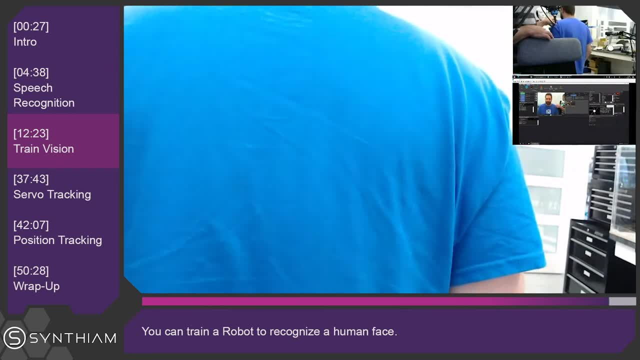 So I don't know. Okay, So, Jeremy, put your face in. I'll tell you where to put your face. Okay, go down a bit, Down Down. Okay, right about there. I know it's annoying. Okay, here we go. 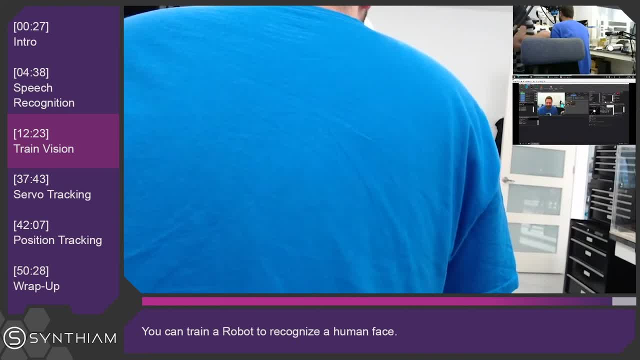 Learn in your face. New object: Okay, what is the name of the new object? Jeremy? Excellent, Let me know when you are ready to teach me what a Jeremy is. I am ready. Okay, I'm going to grab your head, Jer. 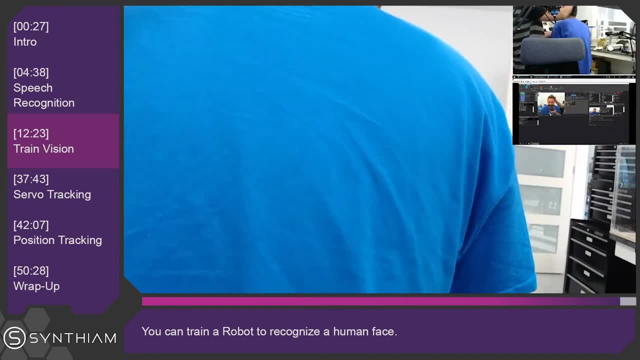 I apologize for this in advance. What if I just tilt it around Because you're not going to be able to know the square You don't know? I know This is so weird. I'm touching Jeremy. This is not social distancing. 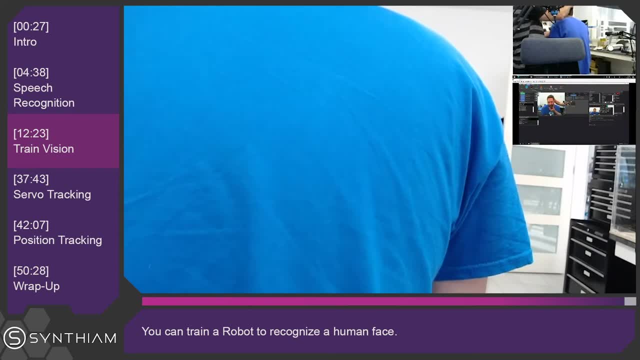 No, Okay, go a little forward A little more. There we go. We want all of Jer's face in the box. That's why I'm having to move forward a little bit And I'm just kind of man-hailing him here. 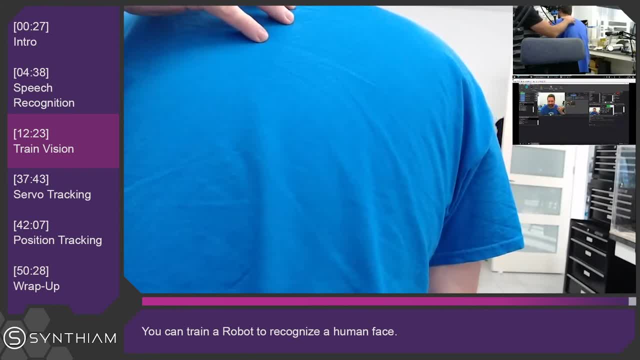 Now smile, Smile Now. frown Looks sad because I'm touching you. There we go. Good face. Well, I don't know if you need that face. Good face expressions is a good thing, And we're almost done, Don't worry. 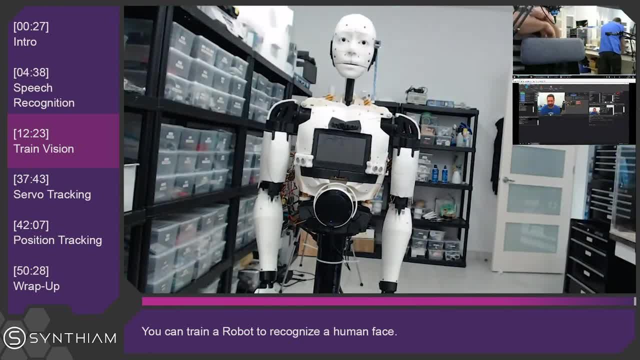 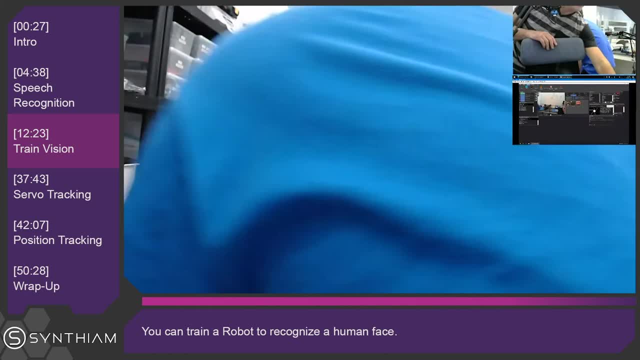 Done There. we learned a Jeremy: Get out of the way. So here we go. So let's put Jeremy's face in front of the robot and see if it remembers Jeremy. I see a Jeremy. It sees a Jeremy. Come on. 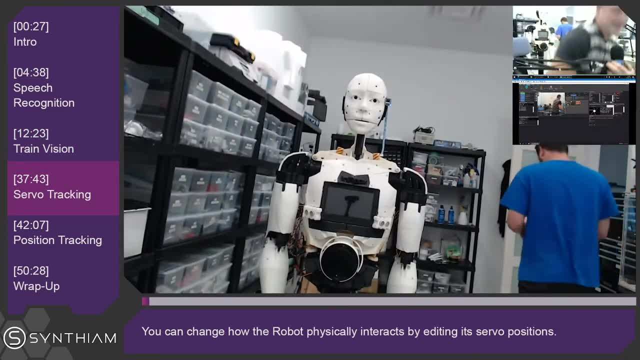 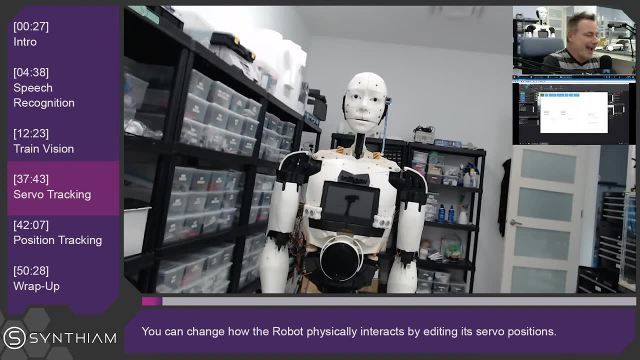 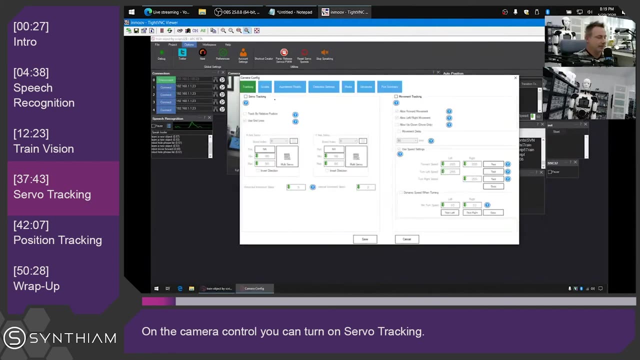 Let's try at least something different than that one position he goes in. So I'm going to go into the camera control and we're going to set up servo tracking with the objects that we've learned. So let's check and make sure our script is not trying to move the robot into a position, because we definitely don't want the robot trying to move right while we're trying to get it to learn something. 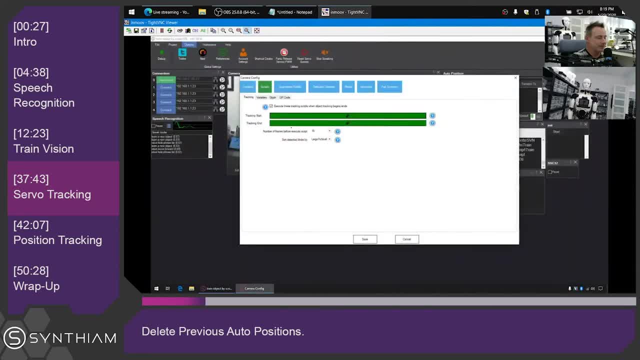 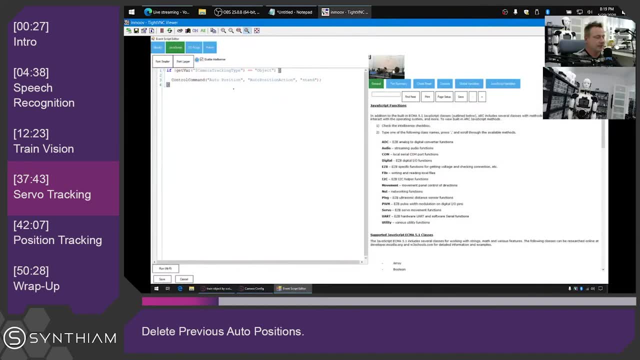 So there's: our auto position has been deleted And our tracking end code. We want to make sure that's empty as well, Because we're no longer going to go into the stand position when we're done. There's no need for that anymore. 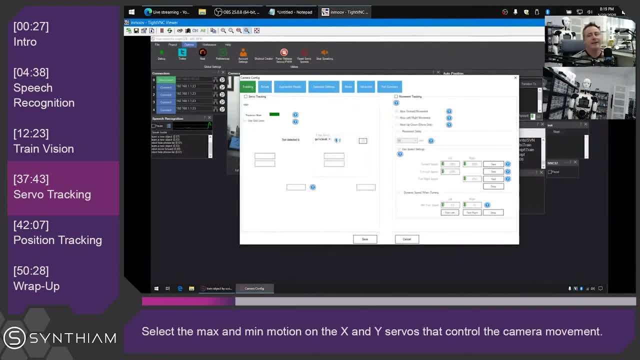 We'll save that And we'll go back to tracking, And in here we're going to turn on servo tracking, And then we have an X-axis and a Y-axis servo, So the camera is mounted into the eye of the robot, which means that we can control its head moving left and right and up and down with the two different servos. 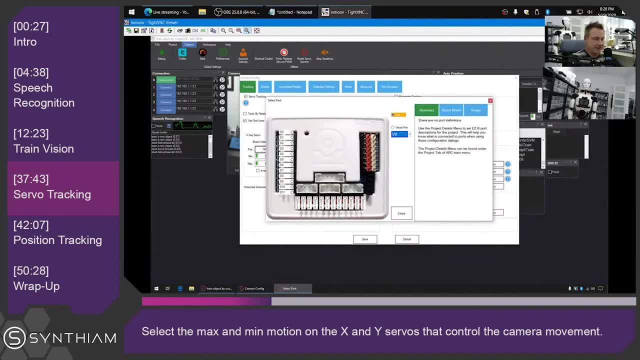 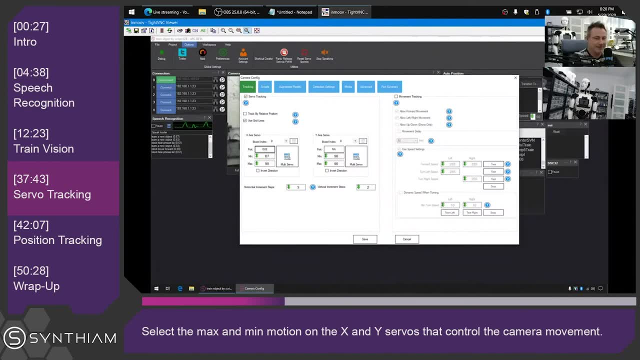 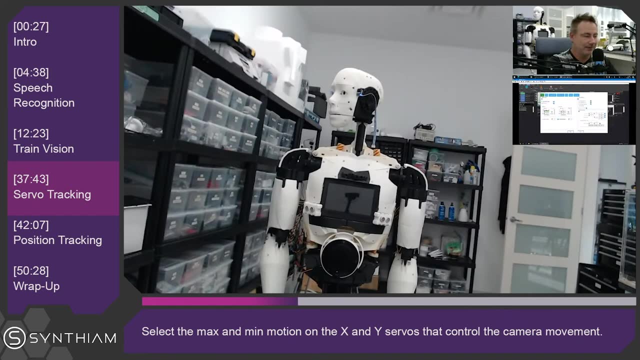 So we'll click on the board Board port for X-axis. So let's see what happens when I move this. Oh yeah, that's moving his. That's moving his head To the left And this is moving his head to the right. 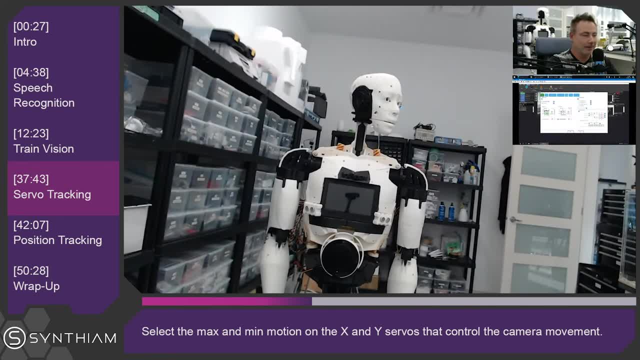 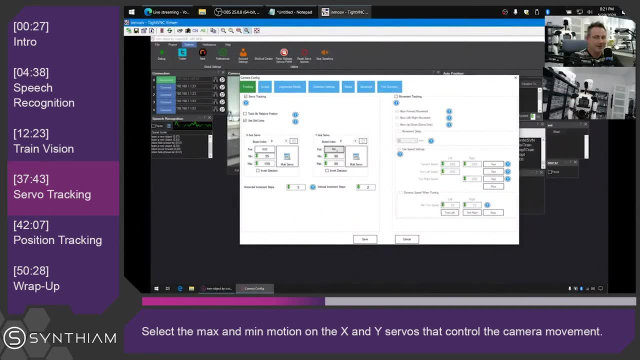 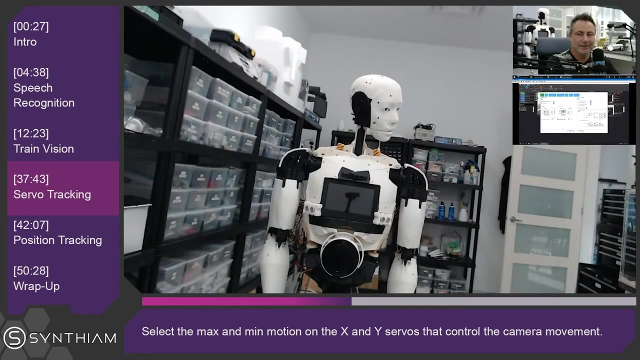 So X-axis is correct, And now we want the Y-axis which, As you guessed, it is going to be 23,. and then we'll have to adjust that accordingly for his up and down. I don't want to burn the servo out, so I know that there's only a certain amount of down. 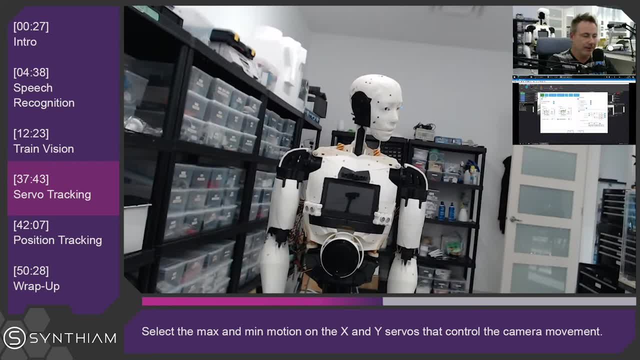 it can go. I think it's right about there- and then up. If it goes too high, then that little neck piece that you can see that's kind of moving up and down there, that piece will pop out. I might have to invert the direction because the max and min, but I don't think. 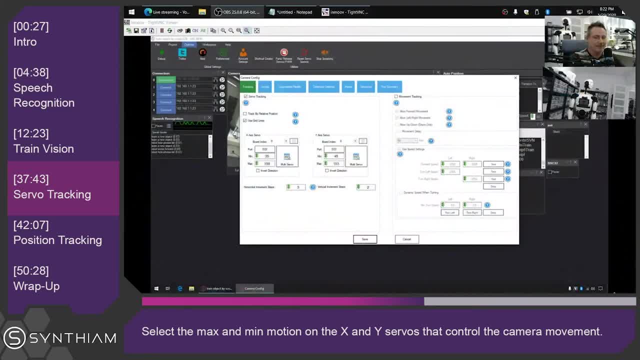 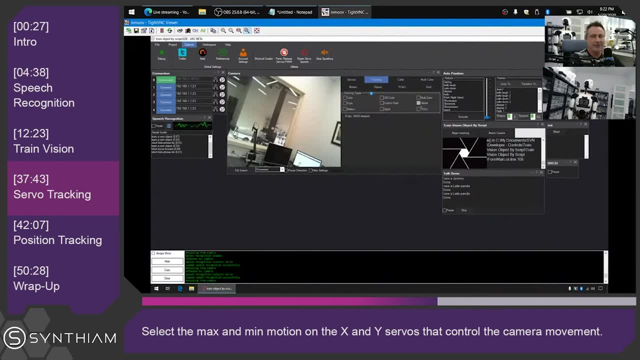 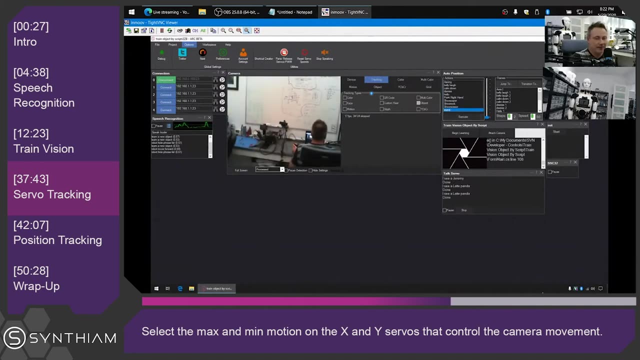 so Let's click save and we'll turn, Turn object tracking on which it is, and then we'll center his head. so I'll just put it into the standing position. There we go Now. let's see if he detects the object and 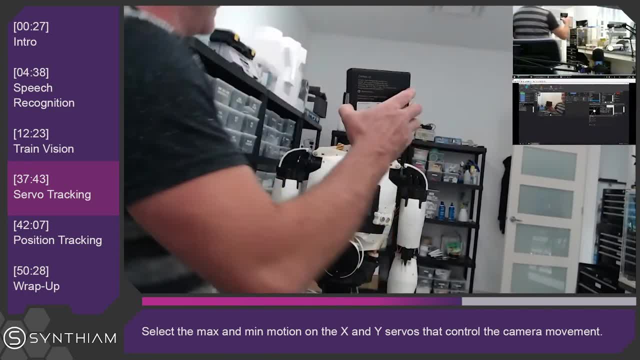 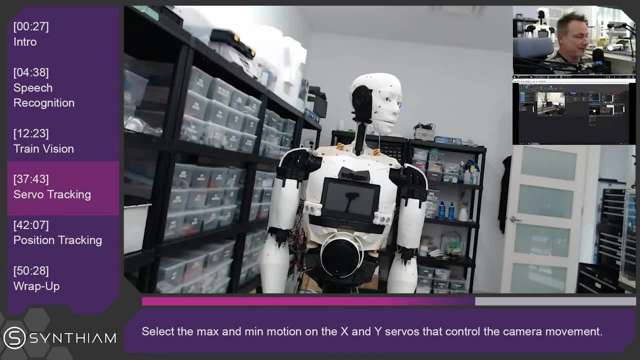 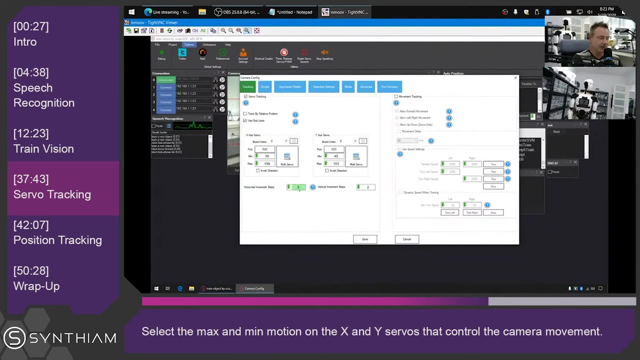 starts tracking it. I see a latte panda. He moved his head far to the right. His head moved really quickly. If we look here, we can see that the horizontal steps are three. We're going to make them one because there's no need for him to be moving his head super. 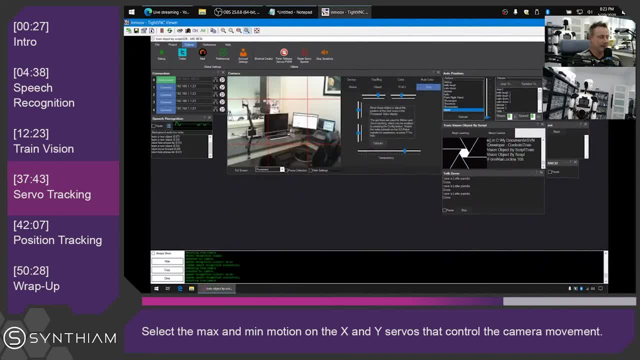 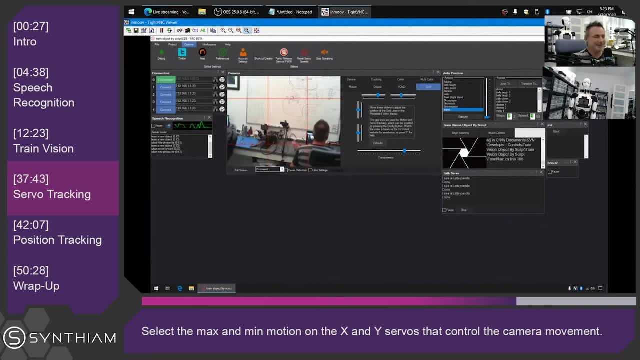 super, super fast. All right, Now let's center his head again, and we also might want to limit how far his head is moving, because it turned really far to the left, so that might be too much. Let's try this again. 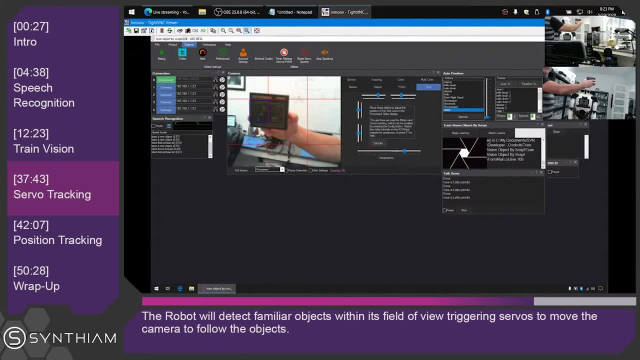 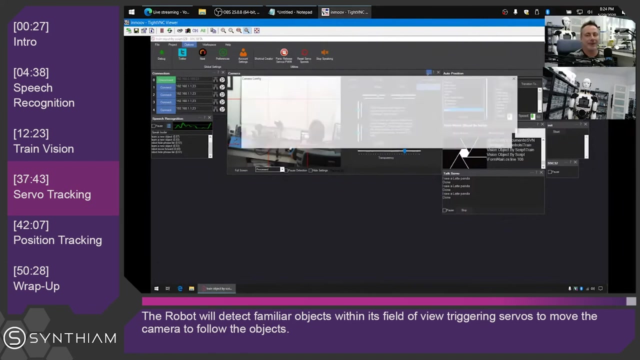 I see a latte panda. Ah, come back. So there you go. That's tracking with his head. So it's pretty good We could tweak it a little bit more. I think one of the tweaks that I would have done if I were going to continue on this. 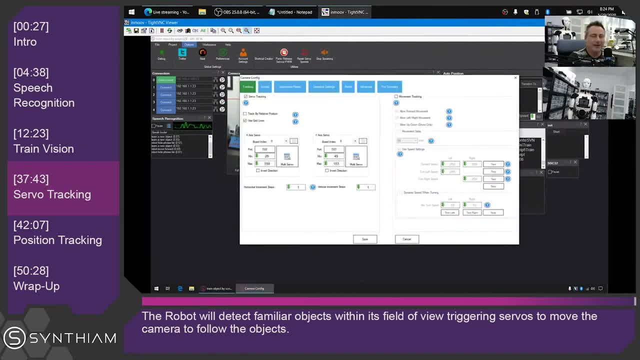 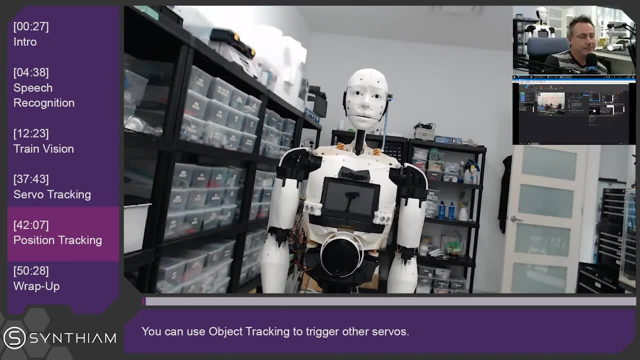 right now is. I definitely wouldn't make his head go as far to the left and right as these are configured. So let me show you something else that can be done. We'll go into the camera tracking, And what I'll do here is set up two switches. 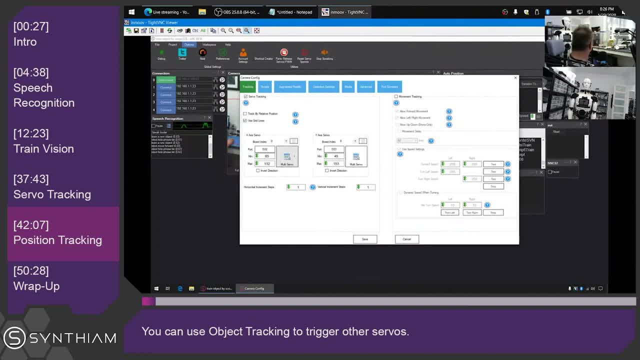 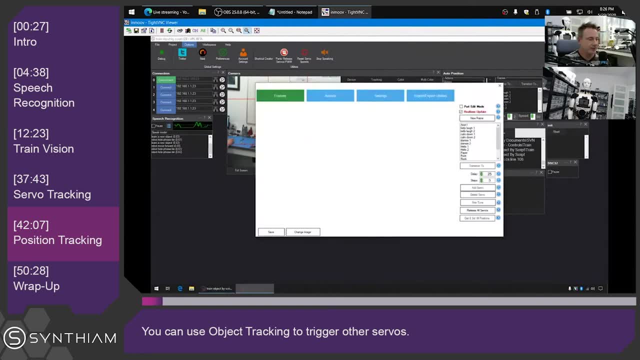 Two servos- Geez, though I don't know what another servo. Let's go take a look in the auto position, because in the auto position that's where the servos are going to be documented, And let's go into the standing position and then we'll go to port edit mode here and 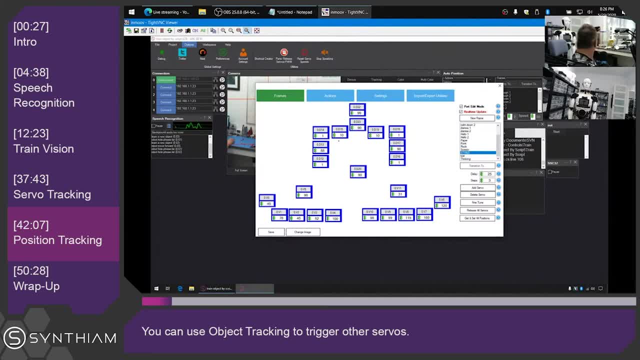 you can see all the servos. So what I'm going to do is I'm going to get his arm, which is this one here. This is his shoulder, It's on D15.. What I'll do is I'll have his arm move up and down. 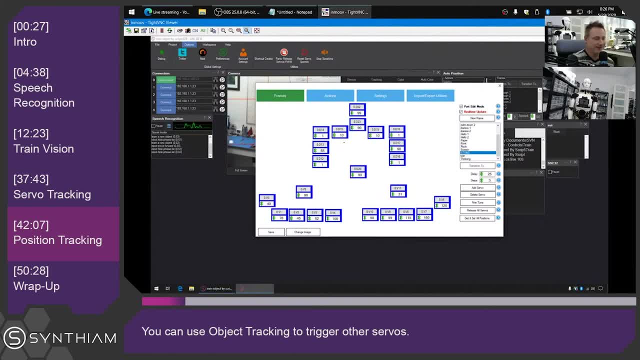 Up and down with the object as it's being detected. Okay, This will be really neat. So D15 is the port we want. Actually, we'll use both. We'll use D15 and D19, and he'll be like a zombie. 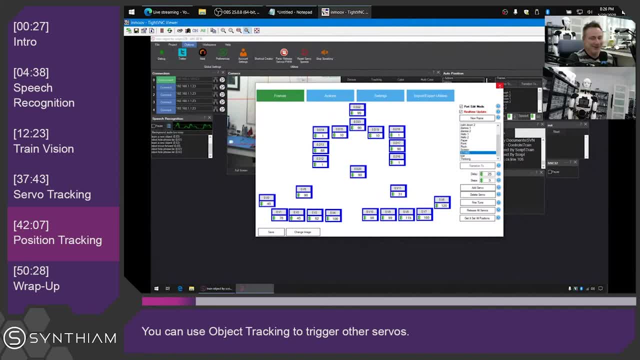 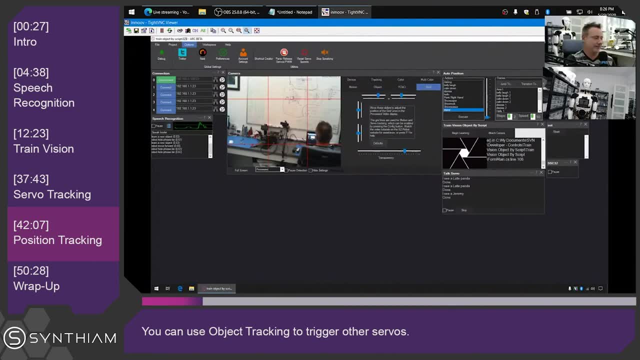 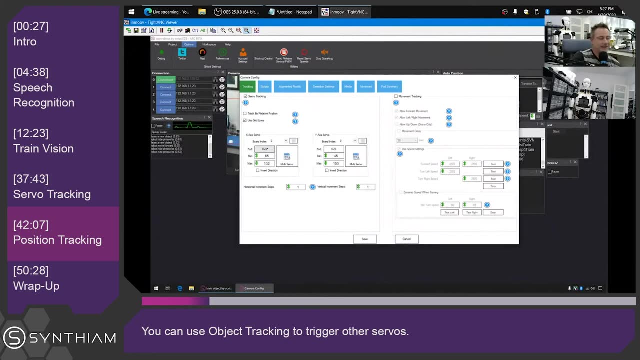 Give me the latte panda, Give me the Jeremy. So watch what I'll do here. So D15 and D19.. Remember those? So now we'll go into the camera and I'm going to turn off the X axis because we don't. 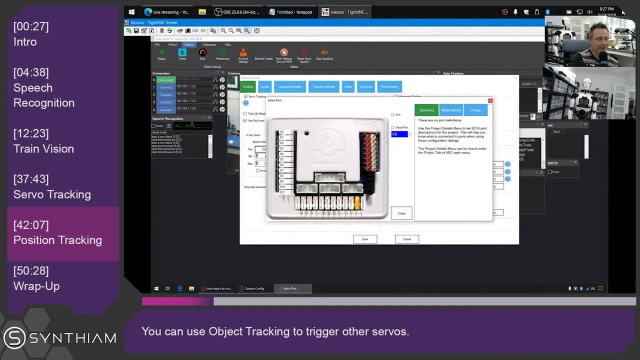 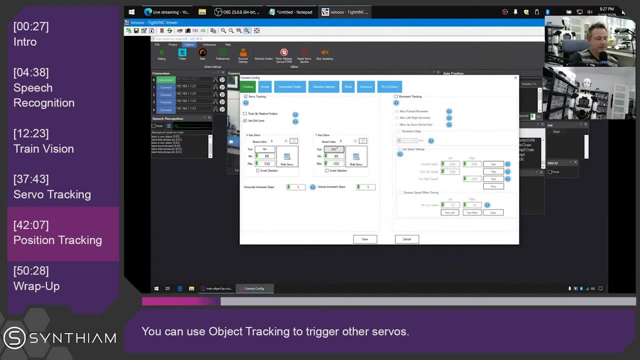 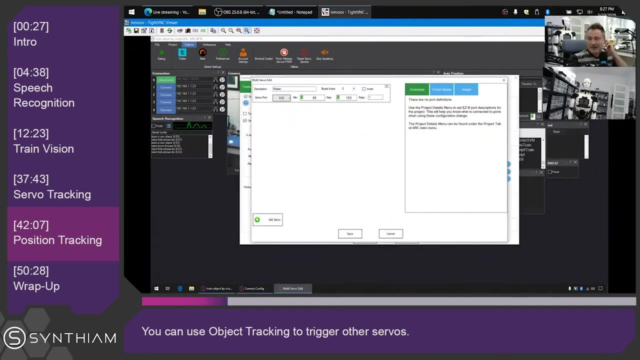 really care about the X axis For this demo, So I'll set it for NA and I'm going to go into the Y axis and I'm going to set up two servos here. I'm going to go to the multi-servo button and multi-servo allows me to set up multiple 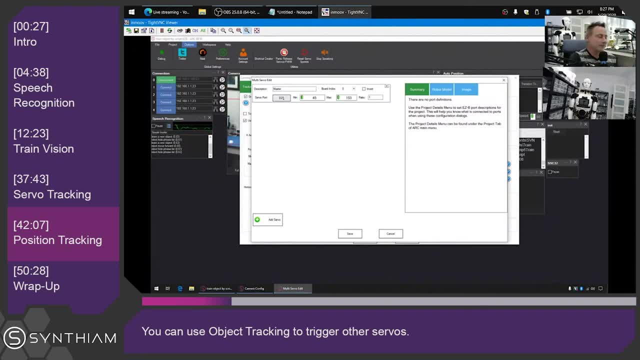 servos that have a ratio of each other, So we can use his head to look up and down, and then what will happen is the arms will be relative to the head position. So I'm going to add another servo here. I'm going to select D15.. 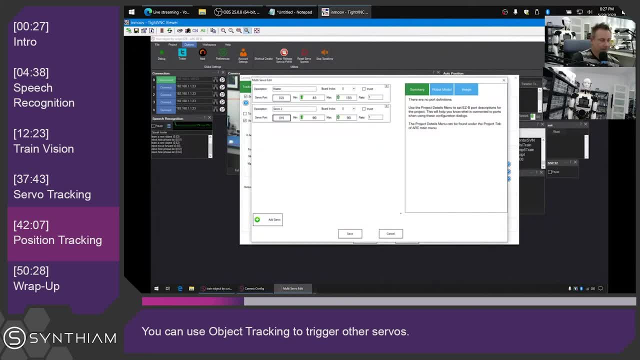 And again I have to specify the min and max position. so it's met. oh, that's the wrong one. That's the shoulders going outwards. Do you see that His arms are going that way like a butterfly, like he's going to fly? 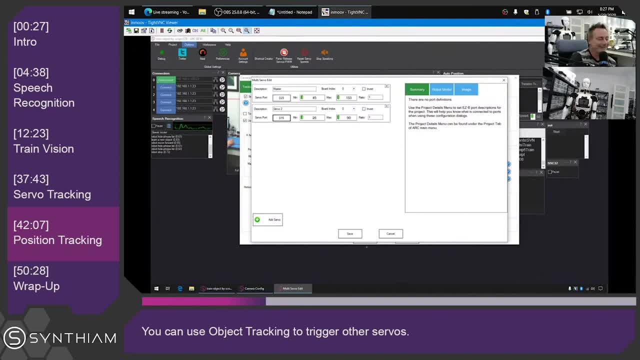 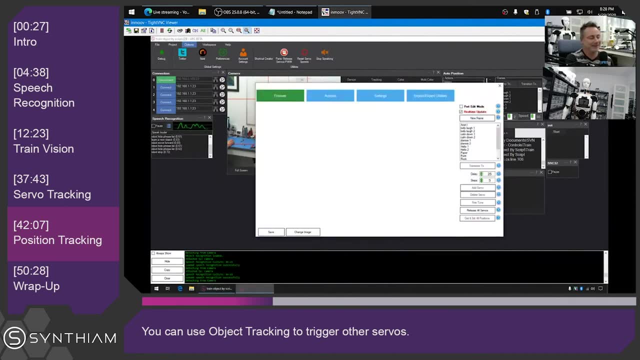 So I don't want that one, I want another servo. Let's take a look, Let's click save And go back in the auto position. I guess I could have just tried. I could have clicked on the servo to see which one it was. 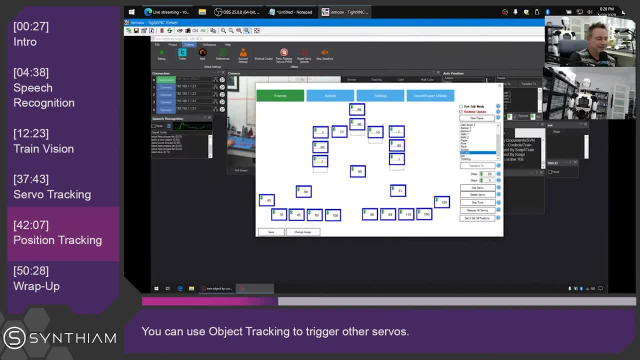 I only guessed. There we go. So servo number this one here, which is number one. let's see, Yeah, that's the one. I can see it moving pointing up now. Okay, So new servos, to remember everyone: D14 and D18.. 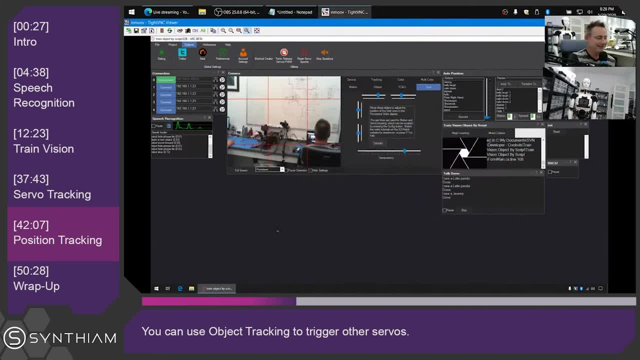 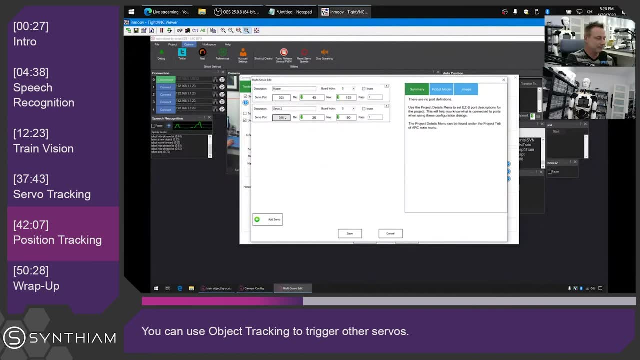 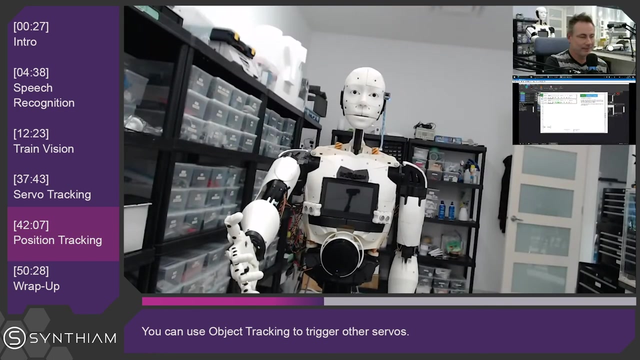 14,, 18,, 14,, 18,, 14,, 18.. Here we go, So go back in here Into the camera control multi-servo 14.. And our min position: we'll bring it up. 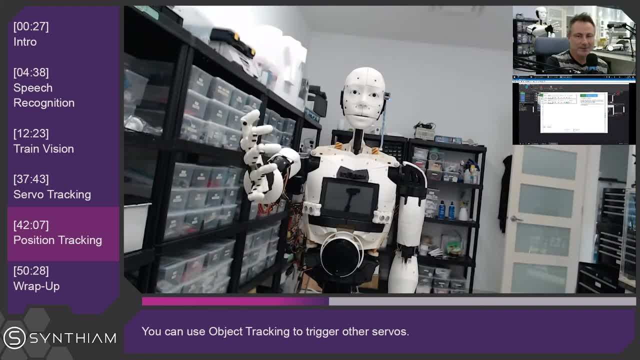 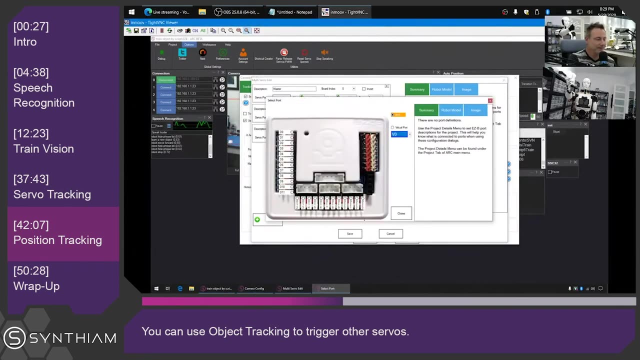 And the max position. this is how high it'll be Okay, There we go, And now we're going to add the other servo, which is just pushing the add servo button, And we'll make this one. what did I say, Jer? 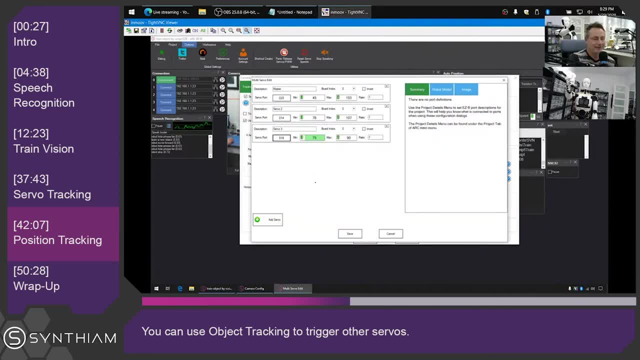 18.. And let's see, if this one I'm failing the test, Jeremy's failing, So we'll do the same thing with this one. We could probably set up similar. Okay. So, first time speaking, we can set up similar positions. 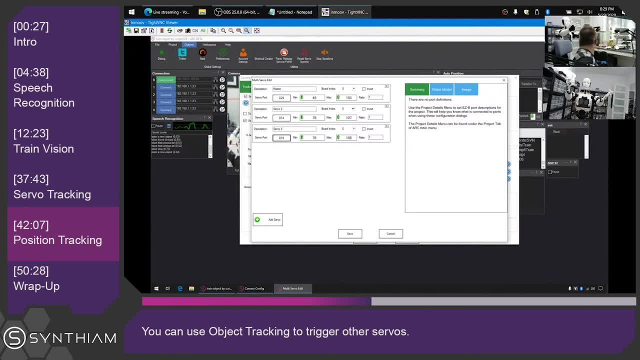 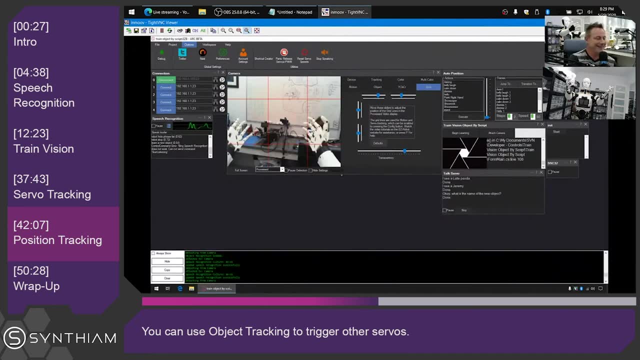 He's very squeaky over there. Do you hear him Squeak? Okay, What is the name of the new object? Cancel, Okay, So he heard me say something that I didn't need to say. Okay, So there's our arms. 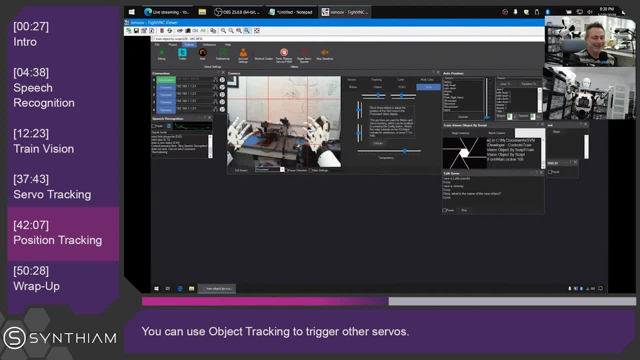 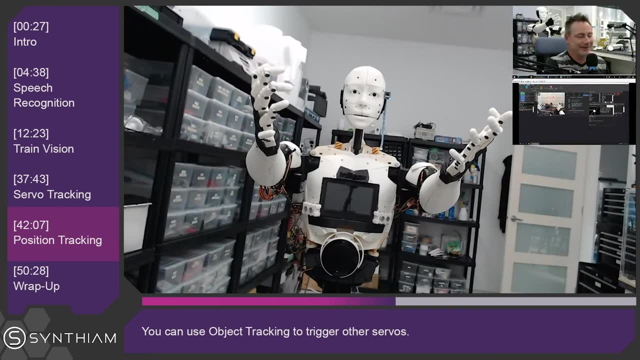 He looks like his. Look at the picture. He looks like a zombie. He's like going to come get you. I'm coming for you. So now that we have all servos set up, I'll put this Latte Panda in front of him. 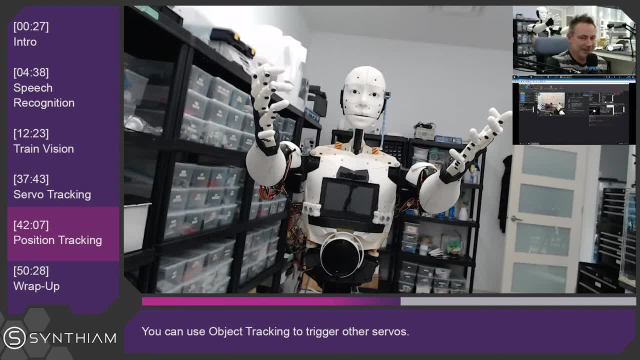 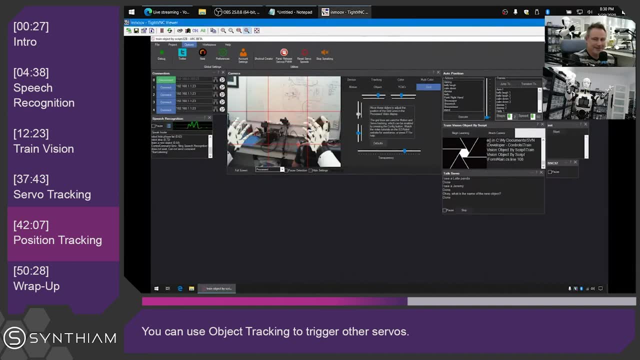 And we can make the robot move up and down. So I'll set up the Here, So I'll set up these grid lines like that, A little bit smaller than they were, And you can tweak these right Like anything that's up above here. he's going to move up. 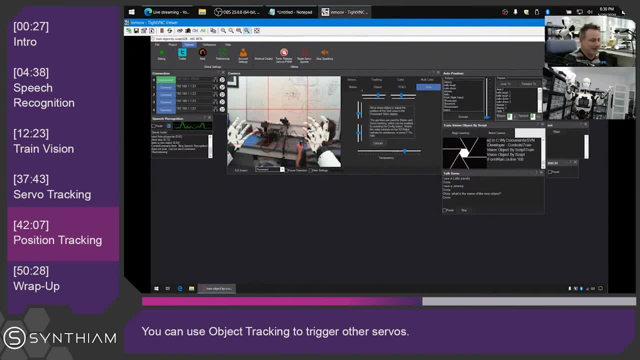 Anything that's lower is going to move lower. So let's see what happens. Go to tracking. make sure object tracking is turned on. It is Okay, Here we go. I see a Latte Panda Come down. I see a Latte Panda. 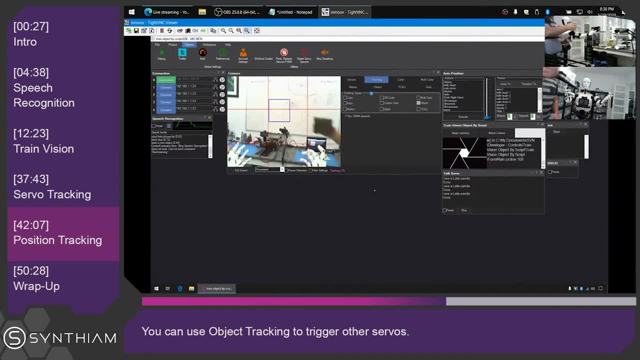 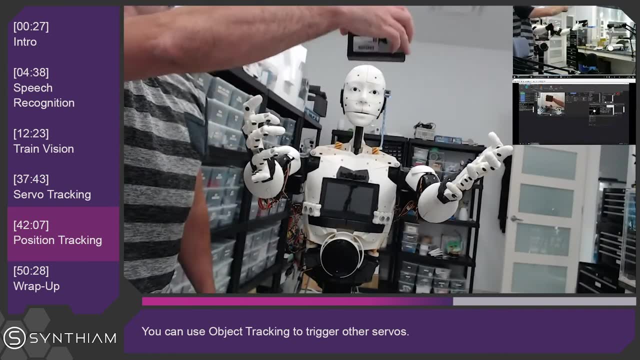 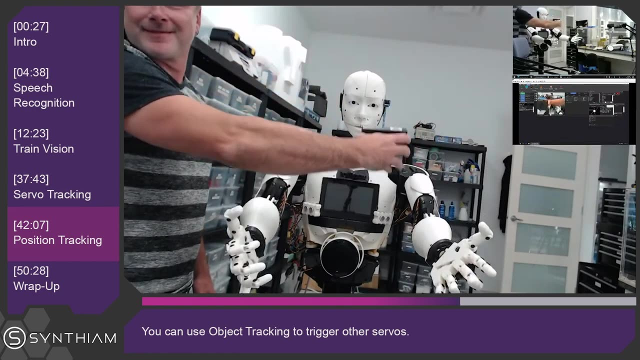 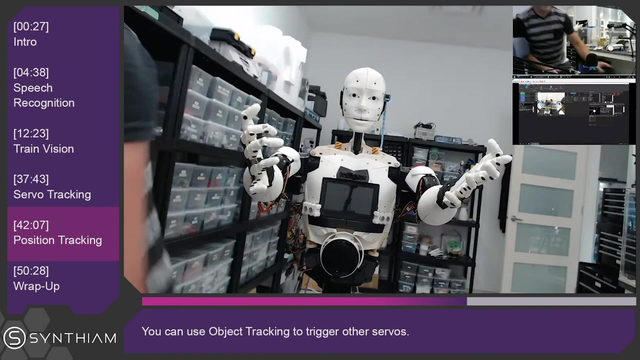 I see a Latte Panda So you can see his arms. here I'll put a bigger screen so you can see. I see a latte panda. There we go. Now. I'll show you one other thing that I just thought of. 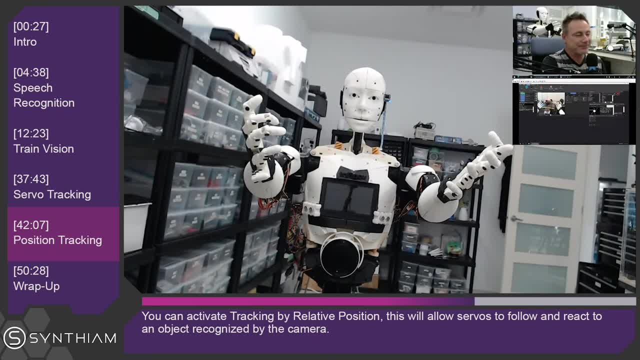 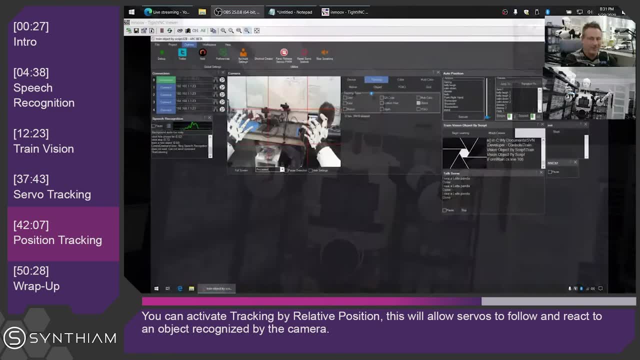 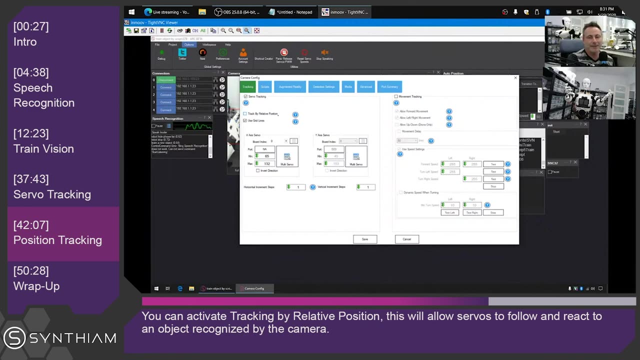 You know how his head is moving up and down with the arms. There is an option in the camera control which I'll show you. That's called track by relative position. You put your cursor over here. it's a lot of wording, but essentially what it means. 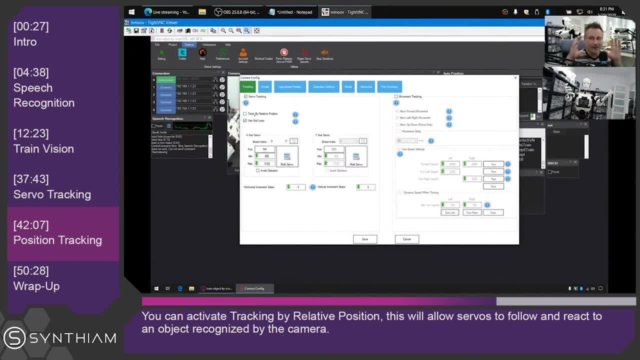 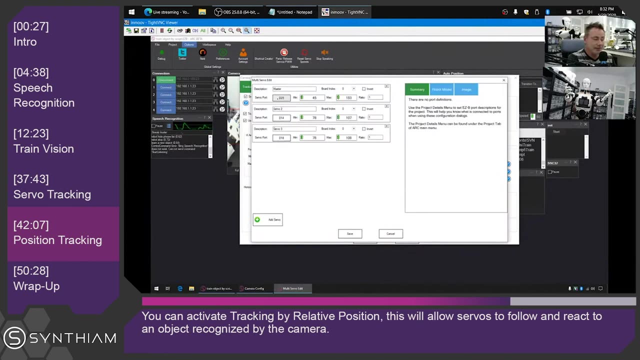 is, the camera is not moving and instead the object that the servo you're controlling is moving based upon, Based upon where the object is on the camera. So if I select this and then the camera is disabled, so this is the camera here, which. 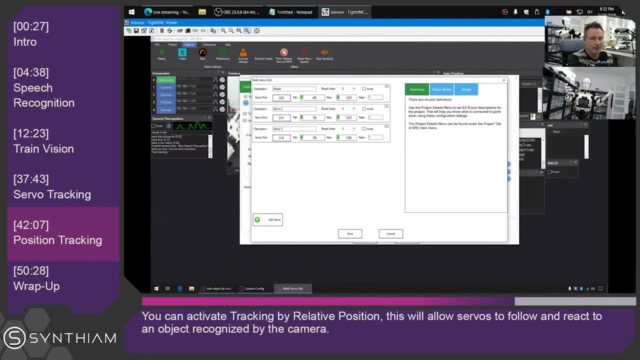 is on D23, let's just remove it entirely. Let's click on this X button Now. the only servos that are here is servo 2 and servo 3.. So for example, here I can type in left arm and right arm, just for future reference. 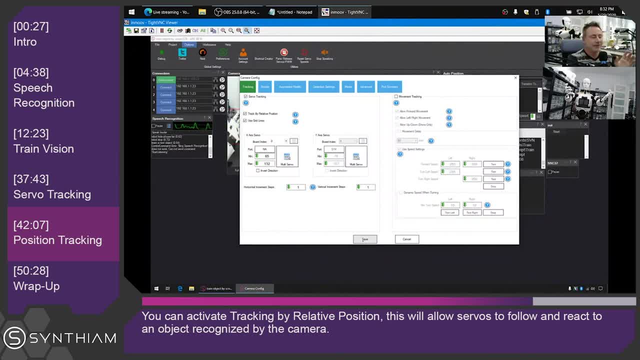 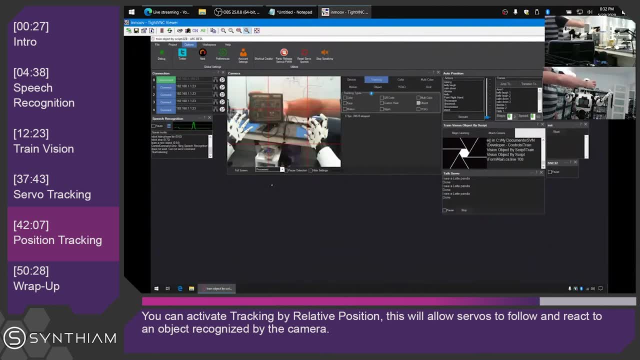 Now what's going to happen is: It's going to stay perfectly still, but the arms are going to move up and down. So I'll show you what this looks like. I see a latte panda Now. I did notice that up and down are reversed. 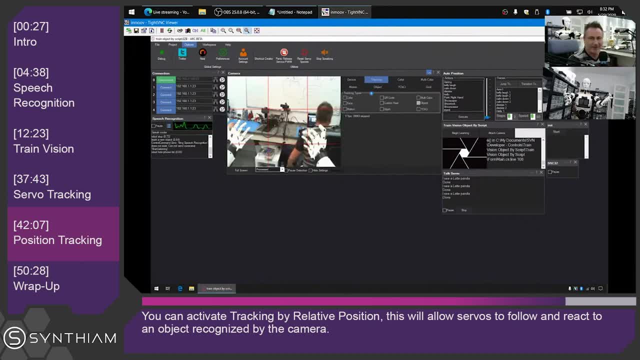 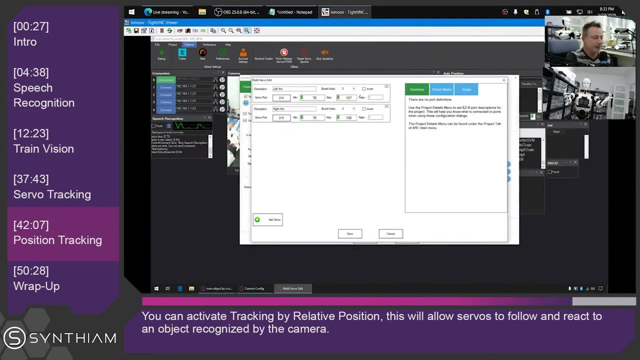 So when I push the object further down on the screen, his arms are moving up. So we'll go back into the camera control configuration and we're going to invert these two servo positions here And then click save. We can also increase the ratio as well. 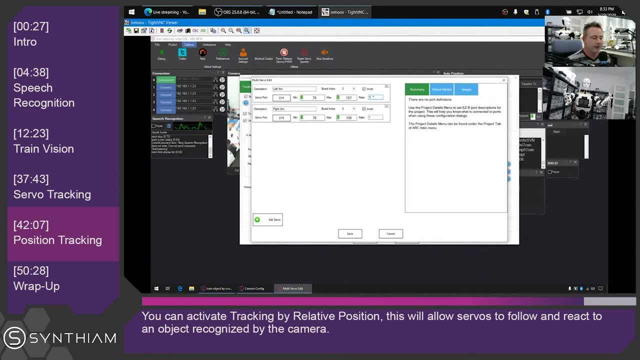 So this means like, based upon um, how many, how many degrees the view actually is, you can make this a larger number, So we can go 1.5, and we can get a larger movement out of the servos, So we can even make it two. 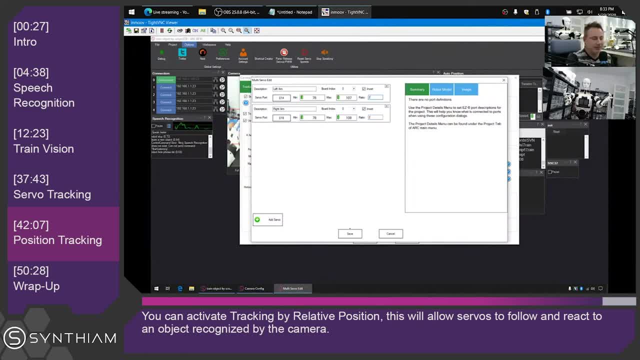 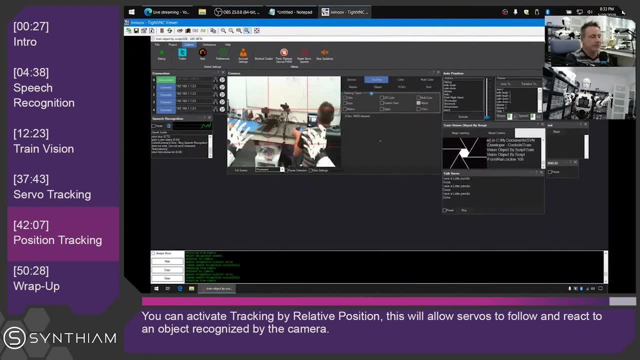 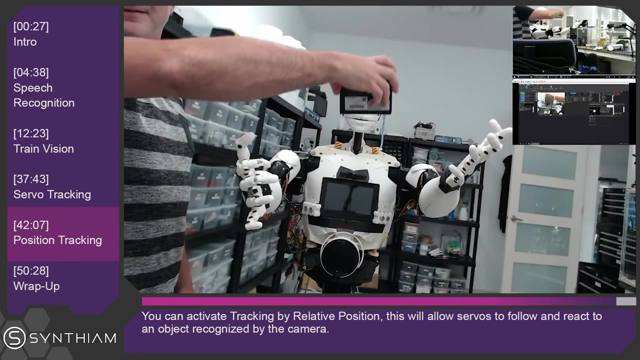 The thing is, it'll never go past the maximum limit, It'll just have a larger. it'll respond with much more. there we go, much more movement. So let me go into full screen so you can see. I see a latte panda.